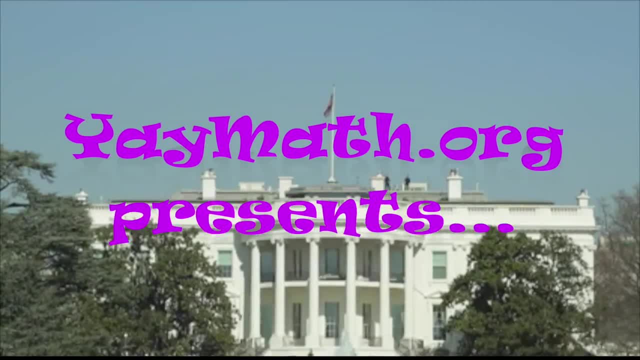 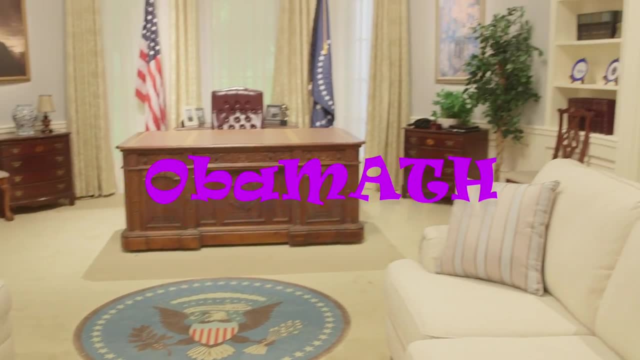 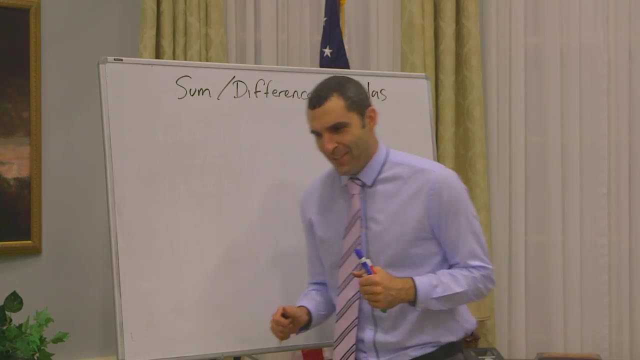 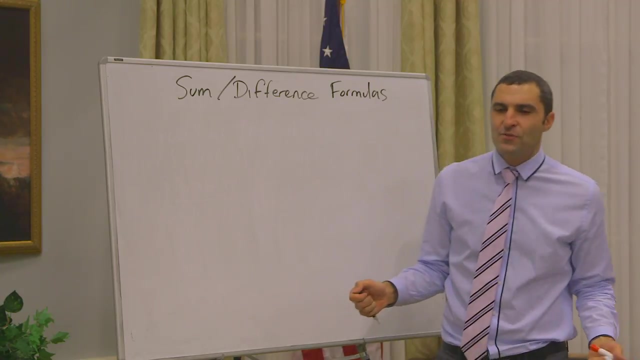 Hello, I'm President Barack Obama, And this is Obama. We're down to two. The other two didn't last, But now we've got twice the energy. Twice the energy. yes, sir, Let's get this going. We're almost out of here, so you can hear a pin drop in the Oval Office. 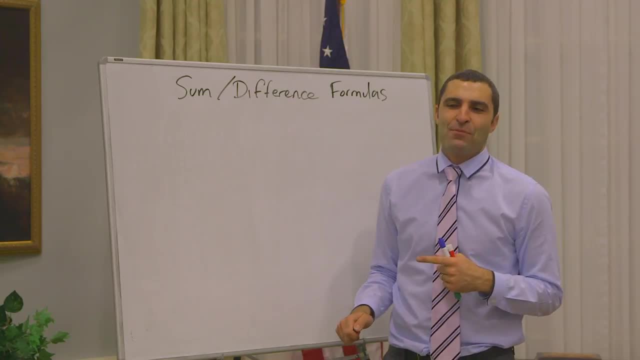 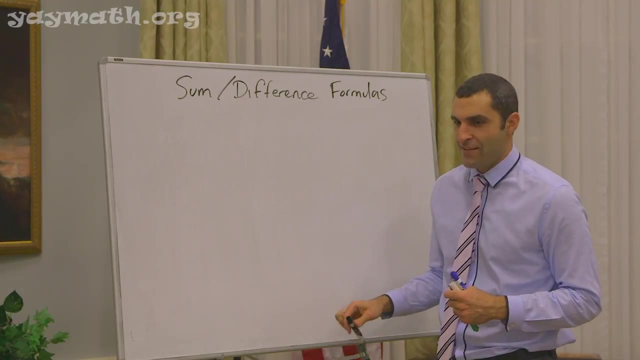 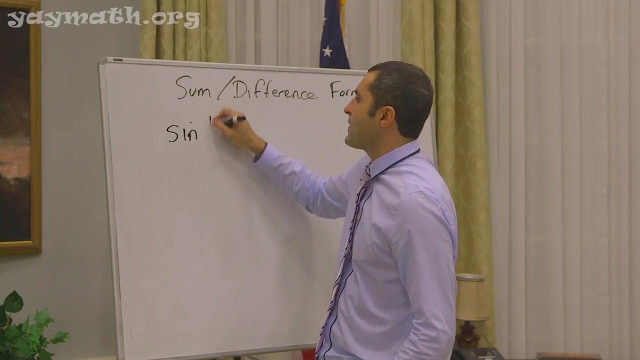 We're going to do some trick, And with my fellow performers, so it's going to be awesome And I mean it. Get ready to sing Like legit sing. We're going to sing. yes, Oh no, Oh yes. So imagine you were trying to do the problem. Sign of, let's say, 15.. 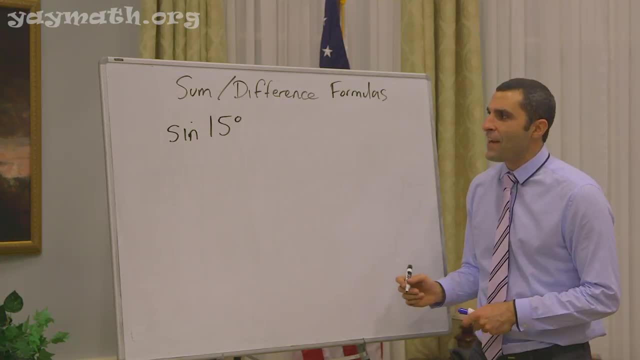 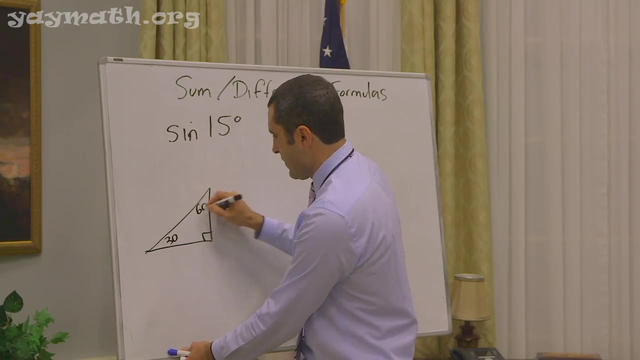 Now is there a 15-75-90 triangle that you know of. Sadly, no, Sadly, no, Hook it up with the 30-60-90.. So 30-60-90, remind me, across from the 30 is. 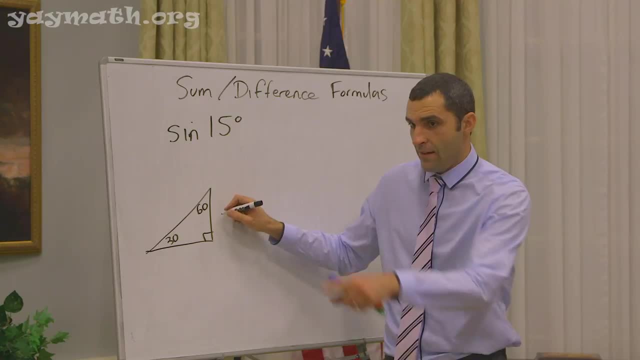 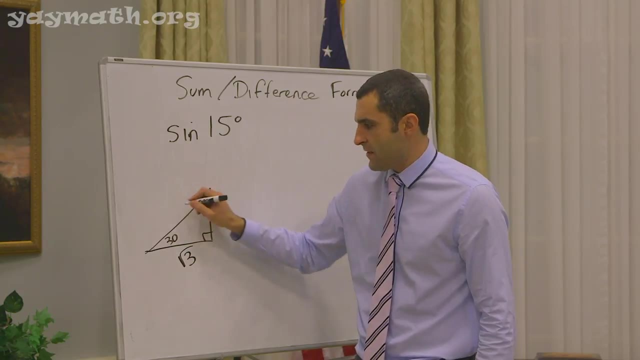 The smallest side. Yes, making it Uh, root 2., Root 3.. Smaller than root 3.. 1. 1. Oh yeah, and then 60 is root 3, and then 2. 2,, very good, 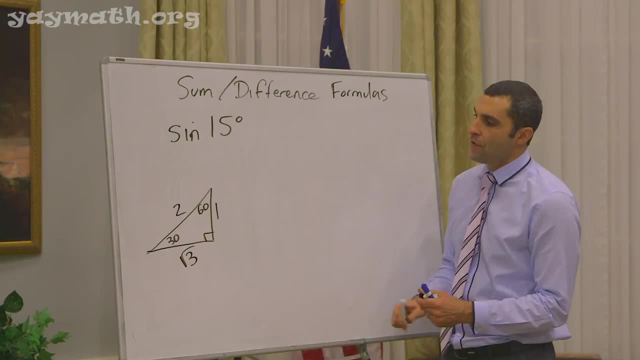 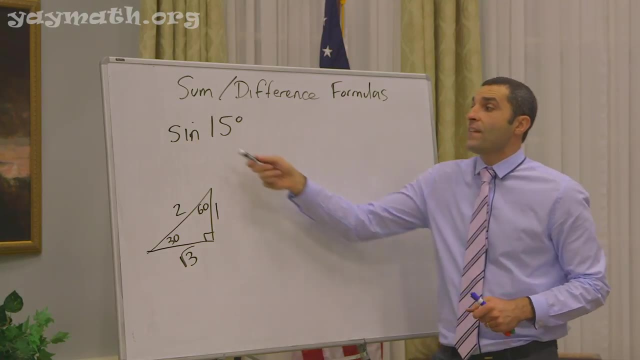 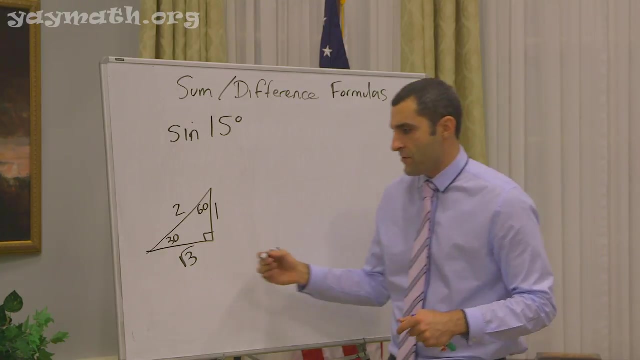 So we can't just say that it's sine of 30 divided by 2, because we're dividing the angle in half. Yes, So we can't really get that situation unless we turn this into a formula. Aw, So let's do the sum and difference formulas for trig. This is how it goes. 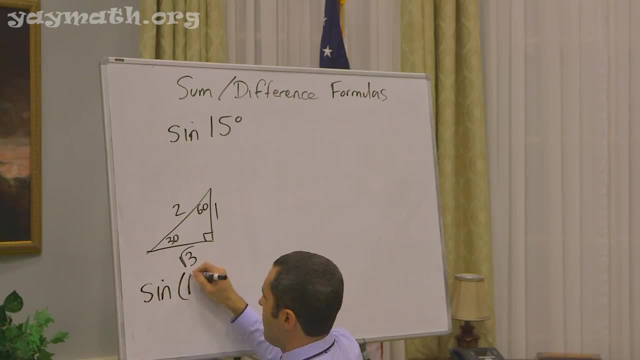 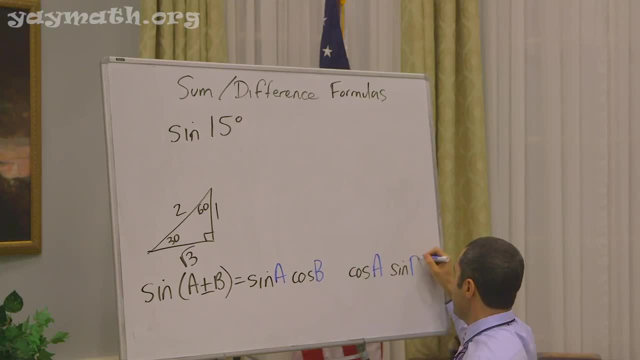 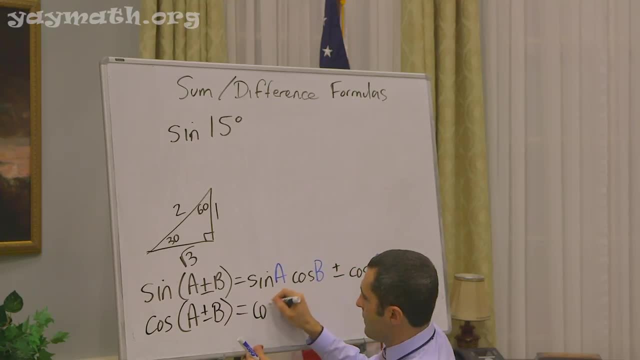 For the cosine formula it's cosine, cosine, sine sine, and again we're going to write a, b, a, b, And you'll notice now, very important, for sine it's plus minus, so it's the same. 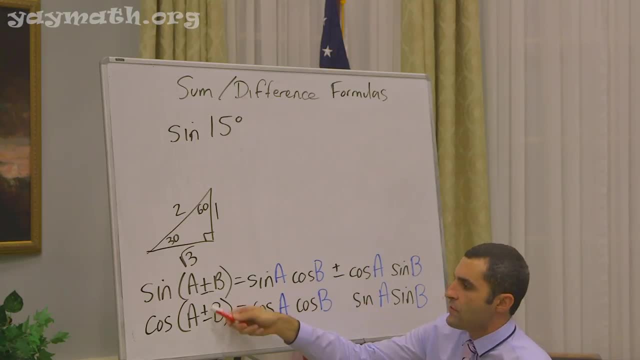 If it's plus here, it's plus here, Mm-hmm, Mm-hmm. If it's minus here, it's minus here, Mm-hmm. For cosine you flip. If it's plus here, it's minus. 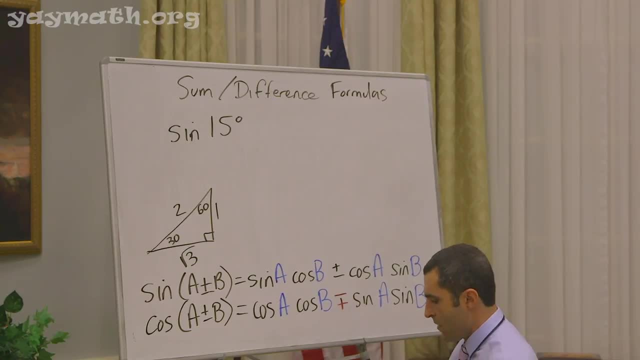 If it's minus, it's plus. Basically, you're going to go minus, plus, like this. Got it Right. Here's how it goes. Oh no, Sine cosine, cosine sine cosine, cosine sine sine. 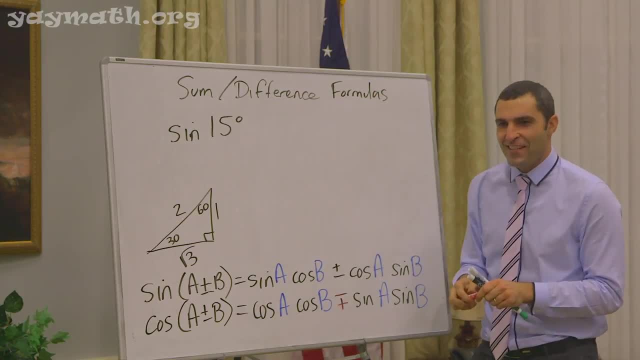 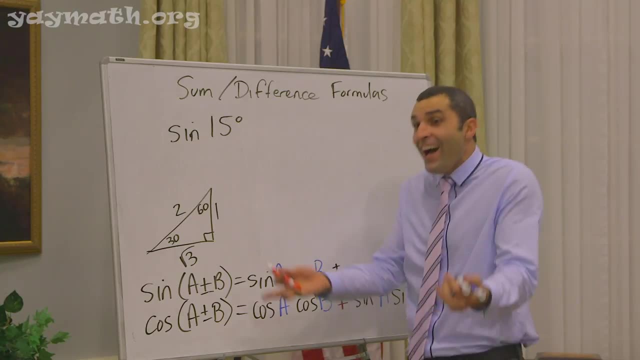 You got to go up. That's my. I added that Digging it: Okay, Want to do it together, Let's do it. Sine cosine, cosine, sine cosine, cosine sine sine Sine na na. 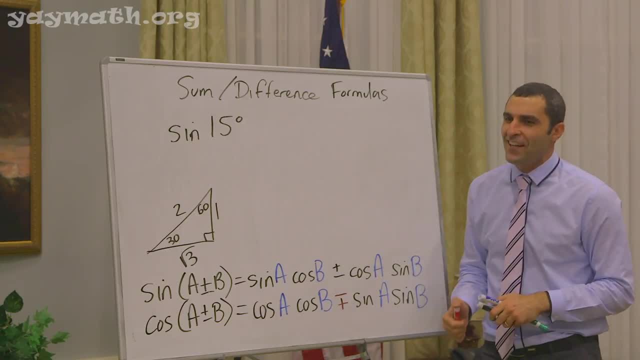 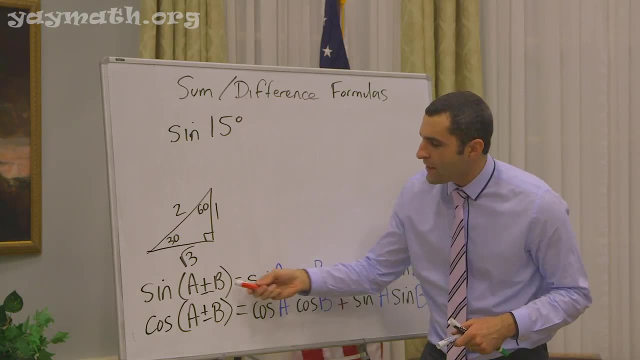 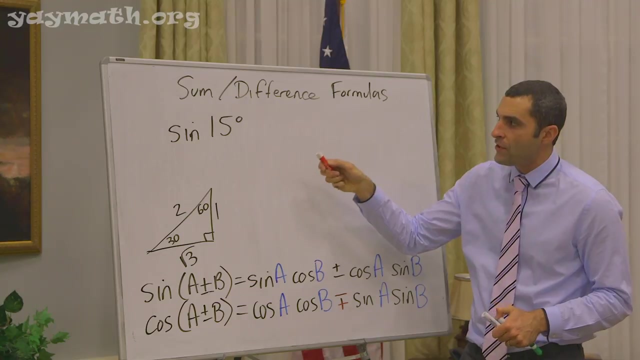 You have to go na Cut off Better training right. Sine na There we go Sine na Done Right. So now we can think of what these two can be as well. So are there certain angles that we can use, either using plus or minus that can arrive. 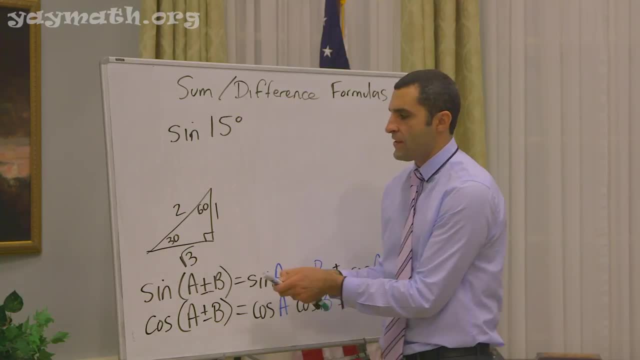 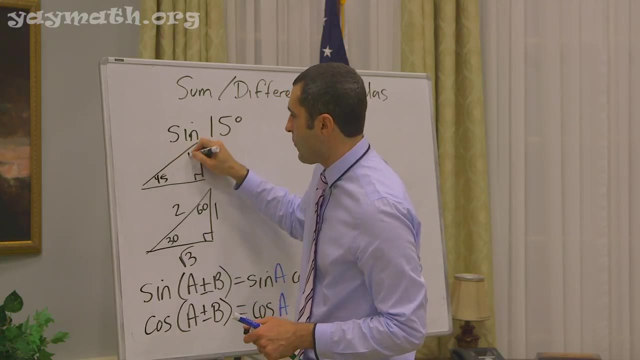 to 15 degrees. I'll give you a hint: It will involve the 30,, 60, 90 and or 45,, 45, 90.. We're going to put it down 45, 45.. Fill me up. 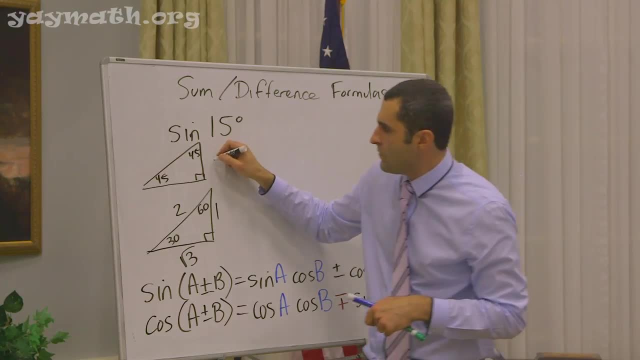 Sides for the 45.. What are the two legs going to be? They're going to be equal. They're going to be one, One and one, Very good. And the hypotenuse Root two, Root, two. What was I saying? 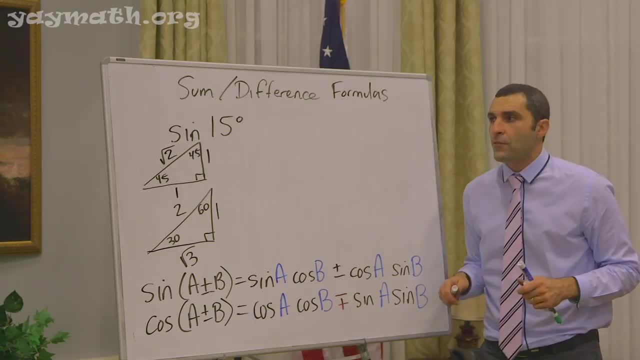 Very nice. Now can you find 30,, 60,, 90s or 45,, 45,, 90s hiding inside, or, to make 15 degrees, Perhaps something plus something or something minus something. I mean 45 minus 30.. 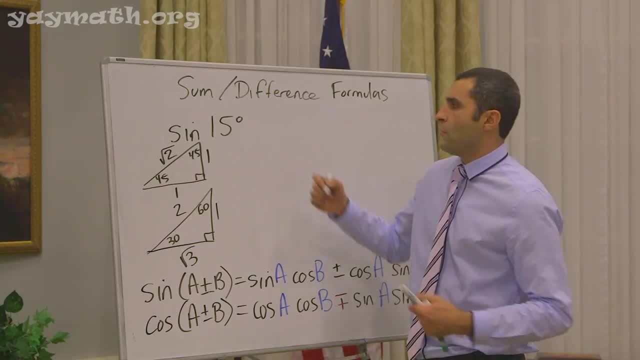 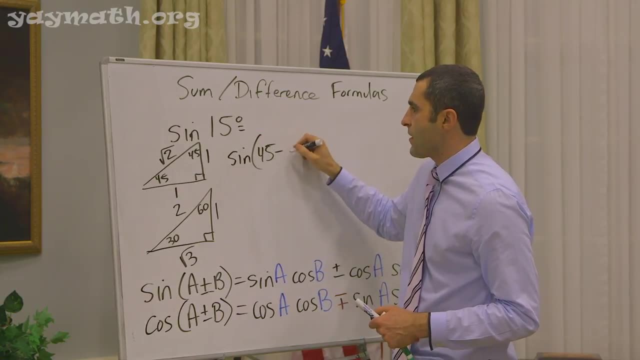 Yes, 45 minus 30 is correct, Yeah, Yeah. So what we're going to do is we're going to call this really sine of 45 minus 30.. Okay, So that is our A and B. 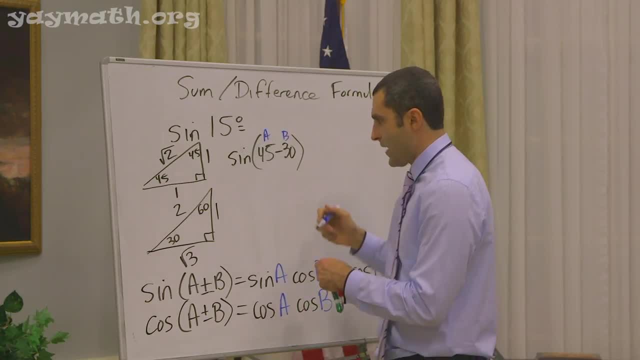 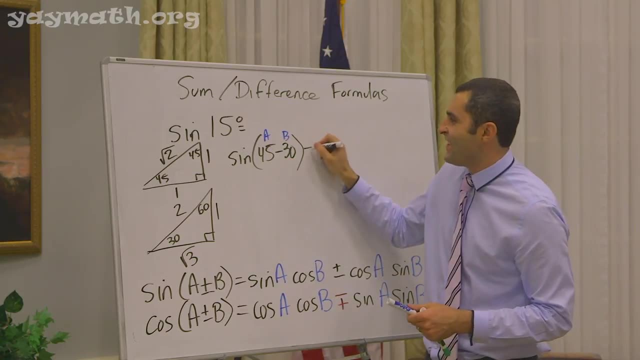 You see it in there. Okay, Awesome, That is our A and D. Makes sense, Okay, Now forgetting about sine for a second, or the negative sine, let's do it For sine. It's sine, cosine, cosine, sine. 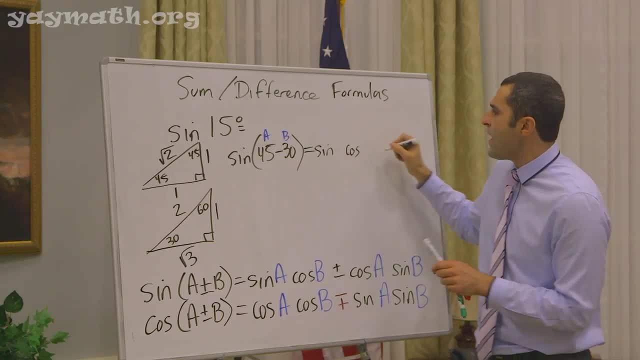 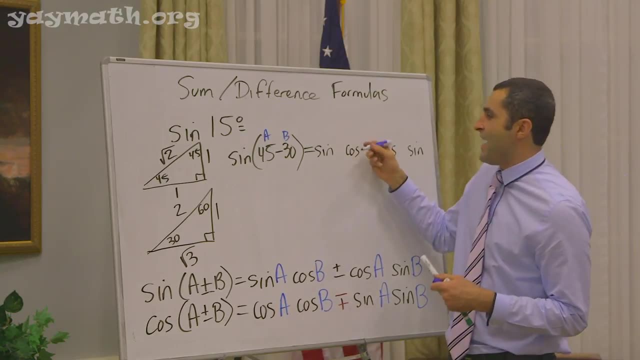 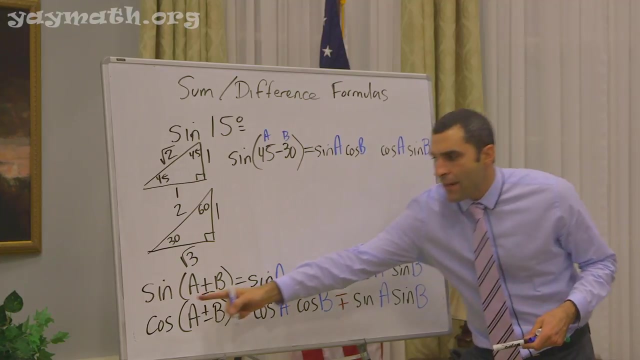 Let's do it: Sine, cosine, cosine, sine. Oh nice riff. Let's put on our A- B. So the good news is, it's always A B, A, B, Five. And now remind me in the sine function: if you have minus here, do you have minus here? 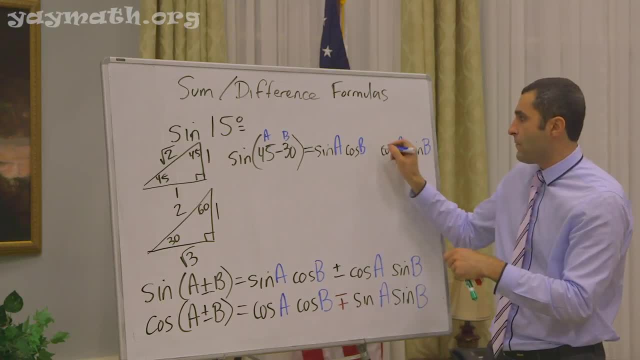 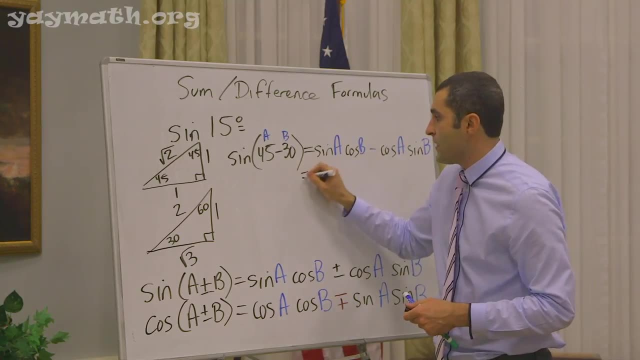 Are they the same? They are. We'll put that minus in there too. Boom, Now that we've established the A's and the B's, let's go ahead and put their numbers. So that's really sine of 45.. 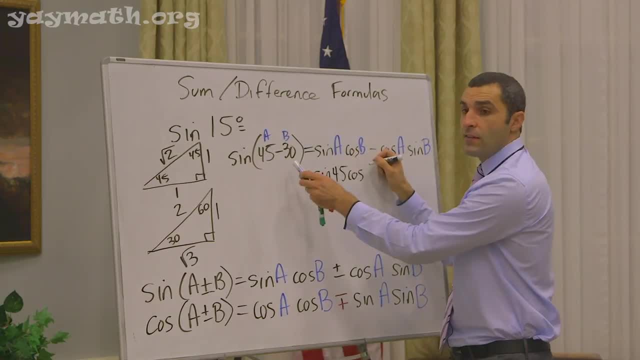 We're good Cosine of 30. Cosine negative 30. Just 30.. Good news for us: The plus or minus is handled within the formula. Do you see that? Okay, yeah, So it's just 30.. 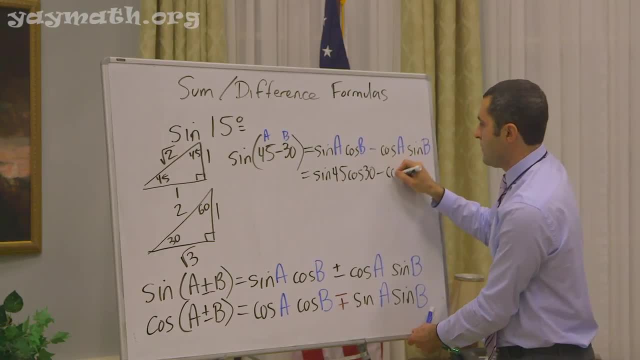 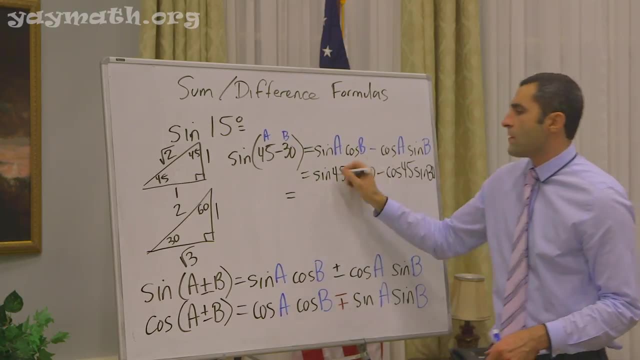 Minus, Minus, Cosine of Cosine 45, sine 30. Excellent, All right, We're going to do these one at a time. Equals Sine of 45 is chilling Right here. Yes, Yeah. 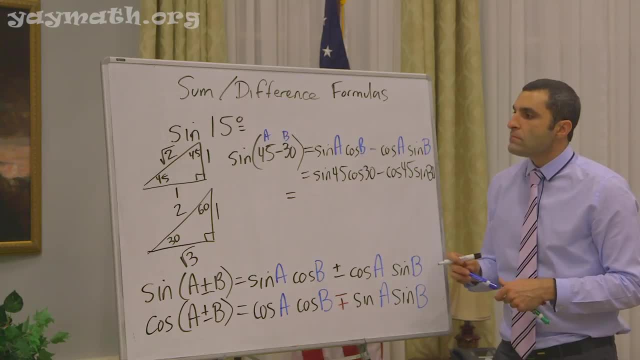 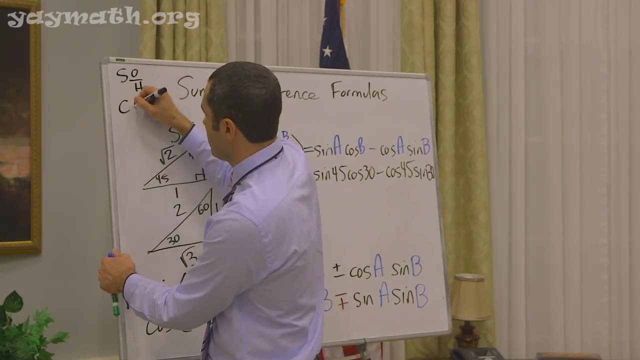 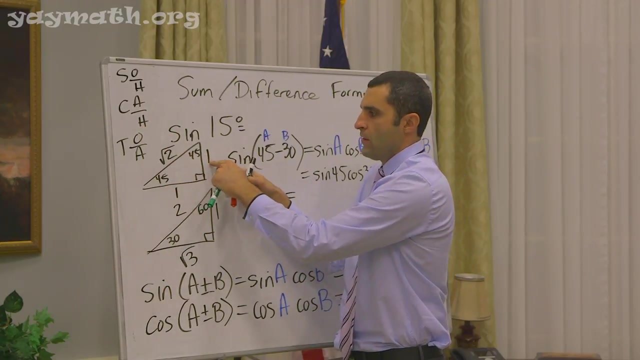 What over what Sine? opposite over hypotenuse. Well done, 45.. Oh my goodness, You got this. Opposite over hypotenuse. Okay, opposite over hypotenuse. So it's one over root 2.. 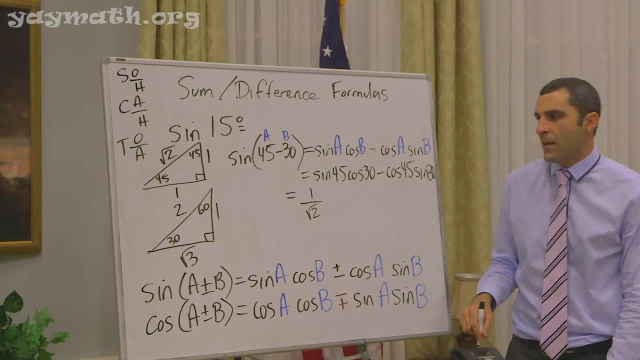 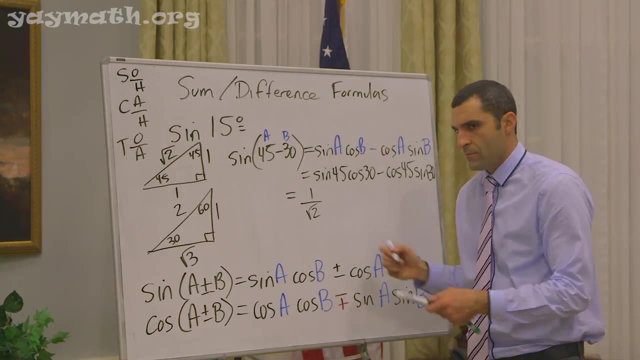 Now here's the thing: Sooner or later, we're going to do this thing where you multiply top and bottom by root 2.. If you multiply top and bottom by root 2, what would you get? You would get root 2 over 2.. 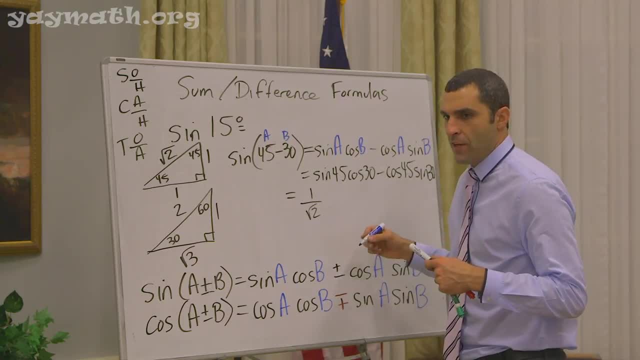 You would, You would. I'm going to do it one time. and now we're straight: From now on, when you do 1 over root 2, it's going to be root 2 over 2.. Okay, Yeah. 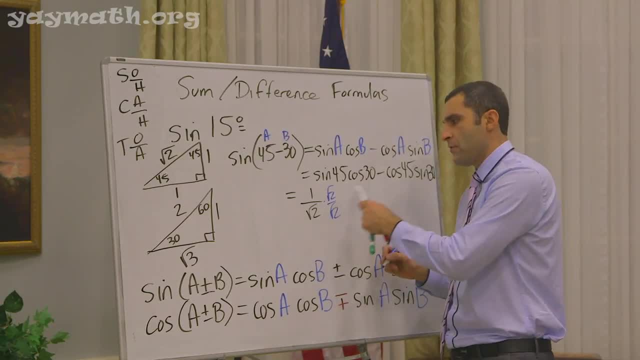 So we got root 2 over 2.. Excuse me, Root 2 over root 2.. Multiply across and you get root 2 over 2.. Do you get that? Do you see that? Yeah, That's root 2 over 2?. 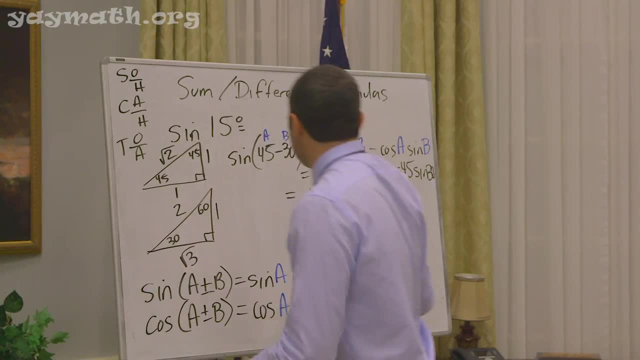 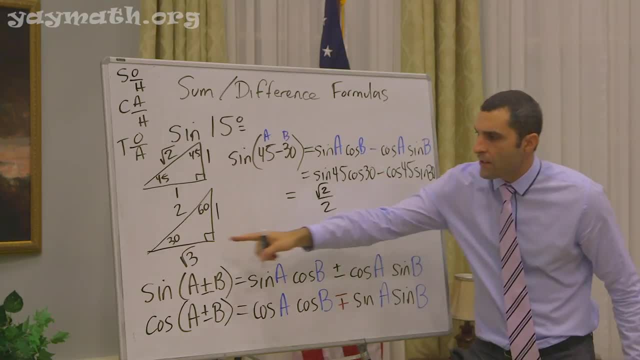 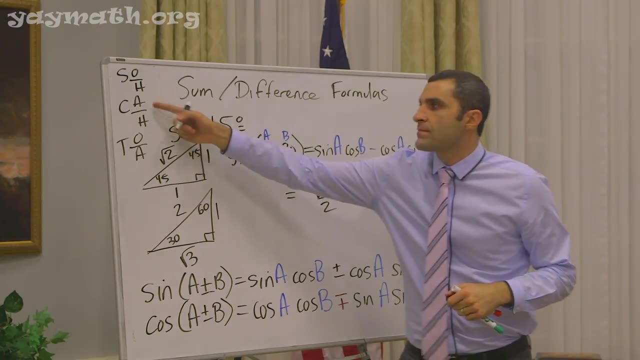 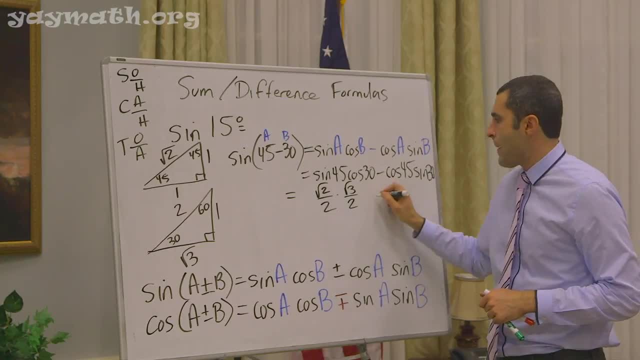 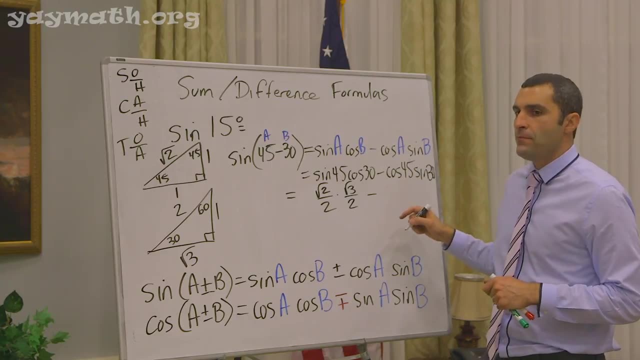 Oh no, It's, It's. It's Root 3 over 2.. Yep, Root 3 over 2.. Very good. Minus: cosine 45.. Minus, So it's 1 over root 2.. 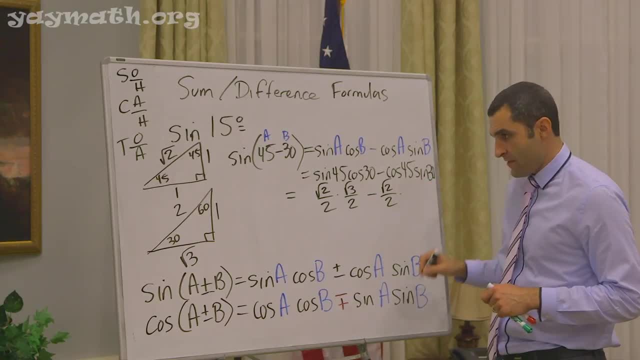 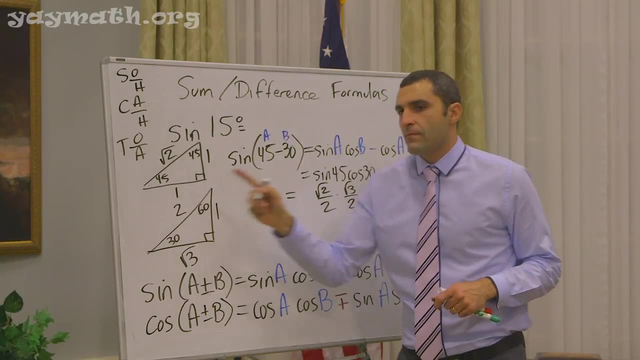 Which simplifies to Root 2 over 2.. Very nice Times sine 30. Here it is, Which is Root 3 over 2.. Yeah, Oh, oh, oh, Which is 1 over 1 over 1.. 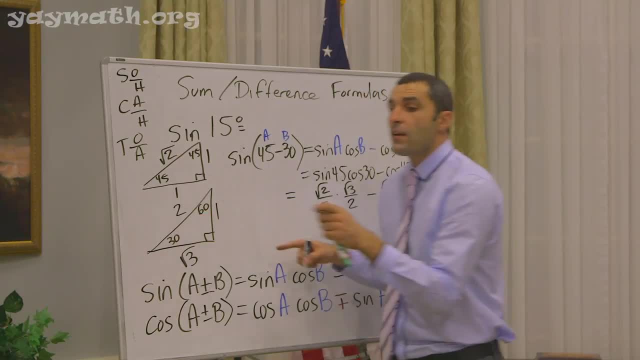 So it's 1. No, 1 over 2.. 1 over 2.. Sorry, Yeah, I looked it up. You know your SOHCAHTOA is just going to be so on point as a result of this. 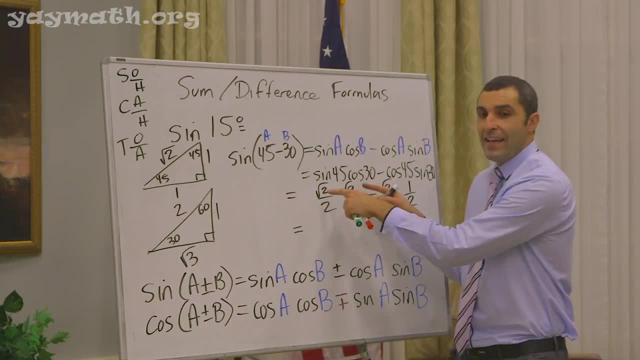 Yes, Very nice. So now, Oh my God, They all have the same denominator. They do. How nice is that? It is very nice. It's going to become one fraction. You're right. Multiply these, What do you get. 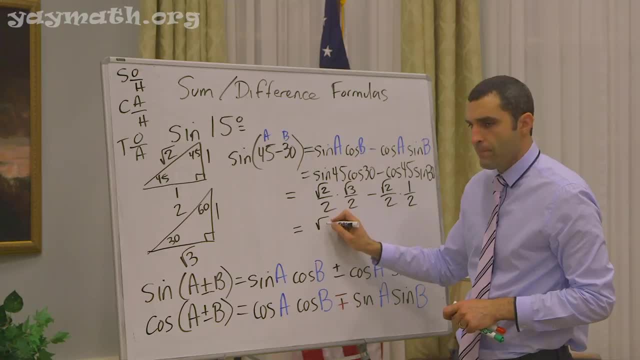 Multiply those, You get Root 2 times root 2 is root. Yeah, It's just root. Root 2 times root 3 is Oh. root 3 is Root. 3 times root 3 is root 4.. 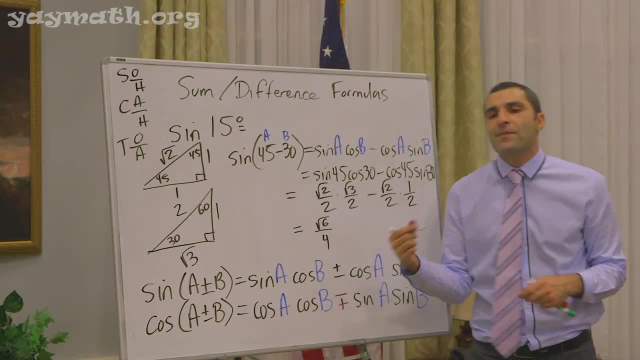 Multiply a fraction. Okay, You're okay As long as you get it. It's okay to make mistakes. In fact, making mistakes is how you get better. It's how you learn from it. If you're not making mistakes, you're not really learning. 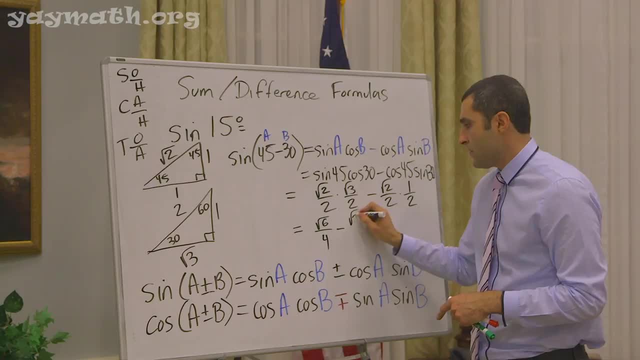 Minus root 2 over 4?? Minus root 2 over 4.. So then you do. Does that simplify? Root 6 minus 2.. Are they? Are we subtracting fractions? Good point, Yes, Yeah. 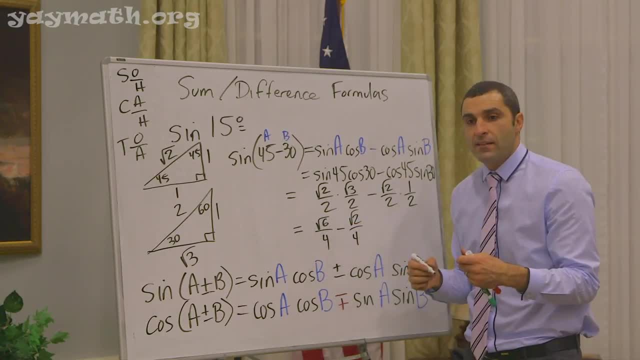 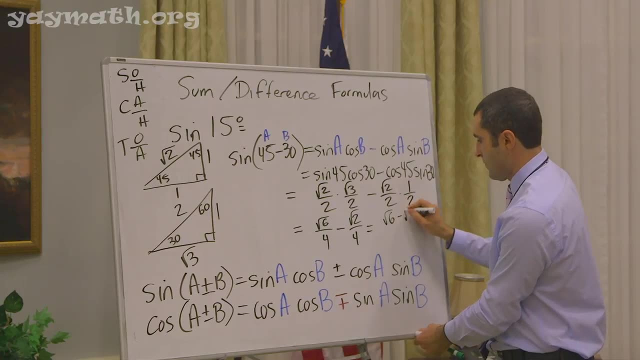 So can we combine them with common denominator? Yes, Yeah, So Are root 6 and root 2 common terms. Do they combine? Yeah, They can, They don't. Oh, no, They don't, They're all over 4.. 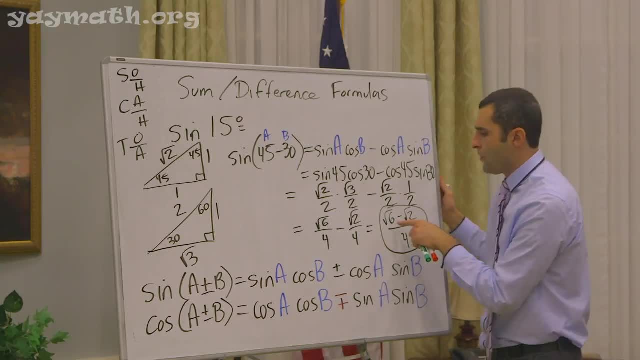 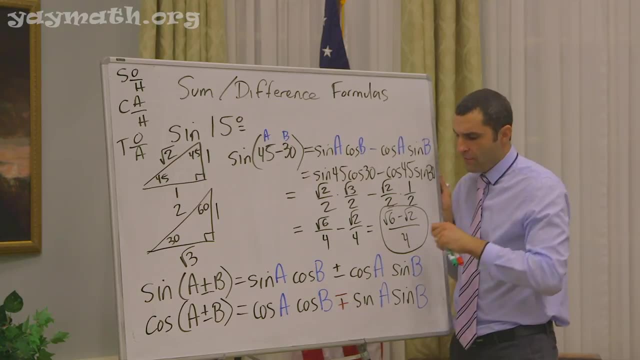 Yes, Right, These are not like terms. Think it through. This would be like 2 point, something forever and ever and ever. This is 1 point, something forever and ever and ever. Very different decimals. The temptation to make this root 4 is wrong because this would not be the square root. 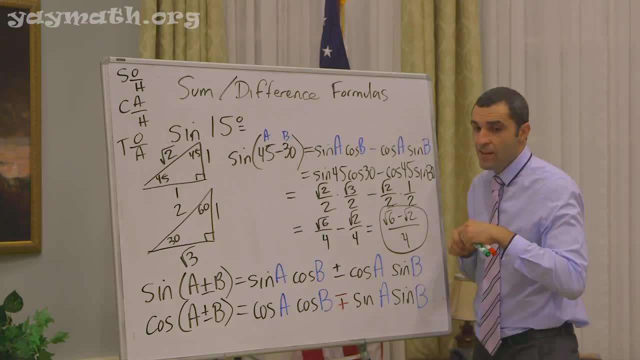 of 4.. Ah, So squares do not combine with plus or minus. Do you want to hear how it gets even better? There's some great news. Let me tell, Just tell me, Tell me, I'll tell you, Tell me. 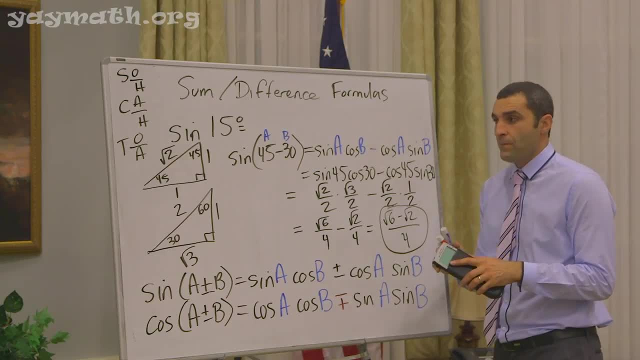 You can check this on the calc. It's really cool. Take a look. Yeah, It's really cool. What I want you to do is open your calc, Go into degree mode, Right, So hit mode. if you haven't. 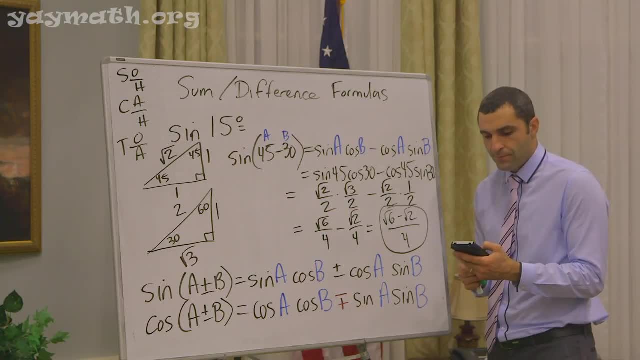 Hit mode and scroll down to degrees and hit enter. Where's my Oh here? Okay, You see it. Yeah, I got it. Hit sign 15 and hit enter. I'm getting .2588.. Yep, Right, Whoa. 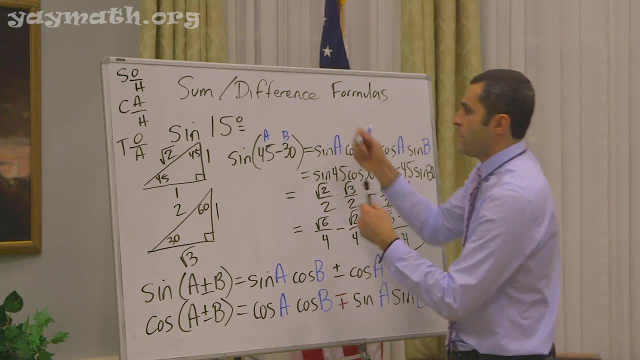 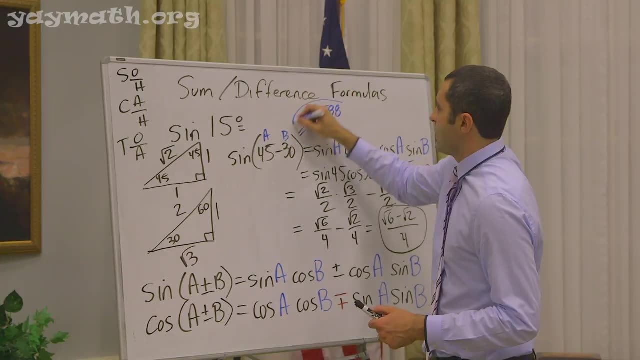 This is, It already came up. Oh yeah, Yours comes into that. Yeah, You have a special calculator: .2588.. And now for you, then Do you? I don't know, I don't know, I don't know. 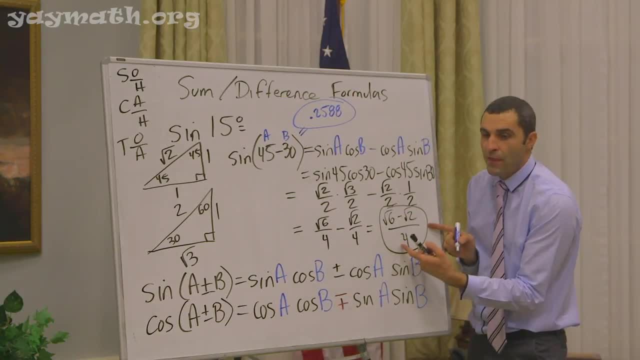 For you, then do you agree that this would be then the same thing? Yeah, Put that in. Let's see if we get it All Put in: root 6 minus root 2, all over 4.. Should I put the mode back to? 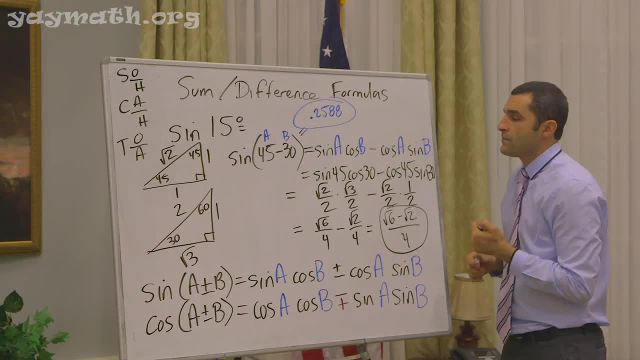 No, Keep it in degrees. Okay, Keep it in degrees Root: 6 minus root. 2. Be careful using parentheses. You might want to hit enter and then divide by 4.. Okay, Enter, You can do that And then divide by 4.. 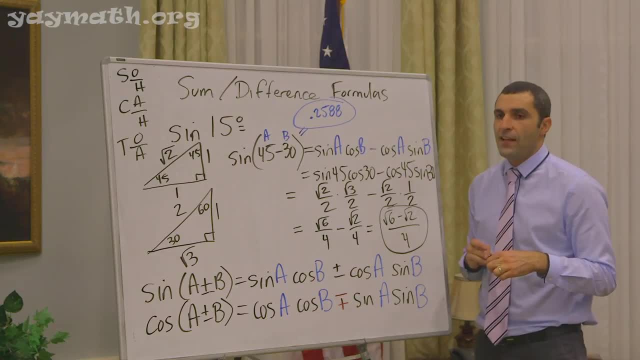 Divide by 4.. Did you get .2588?? Yeah, Yes. So now you know you got it right. Mm-hmm Right. So I'm glad you calculated Done. So this is what it does. 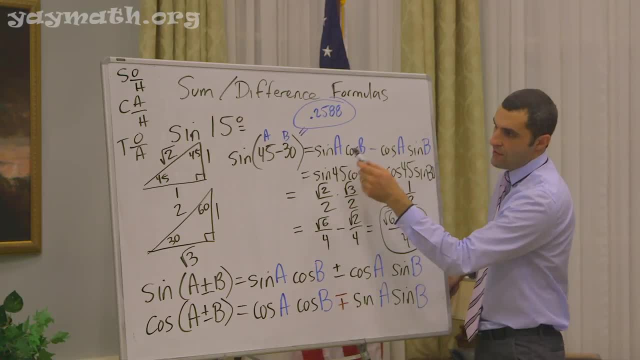 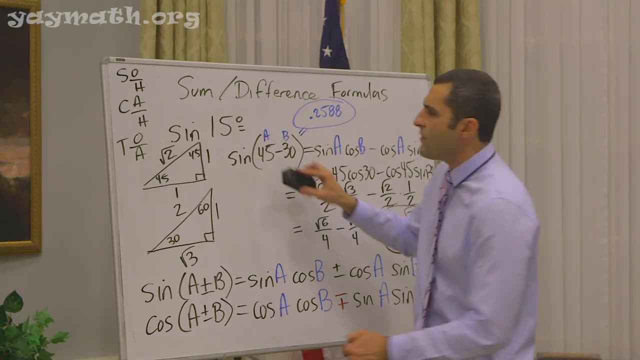 That shows you that thing, but clearly you have to be able to show your work on test Mm-hmm. So this is the process by doing the difference formula for tricks: Ooh Formula, Sine, Cosine, Cosine. 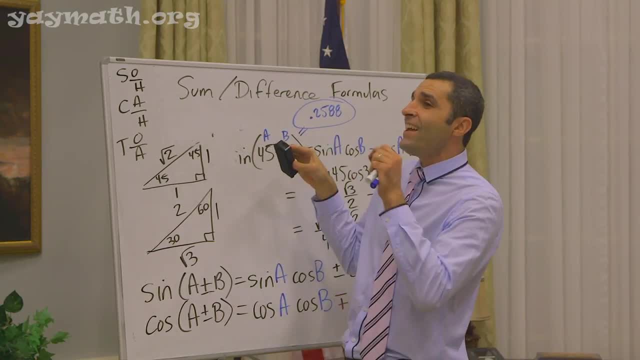 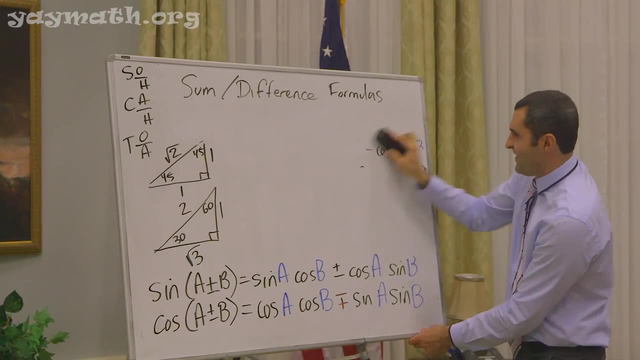 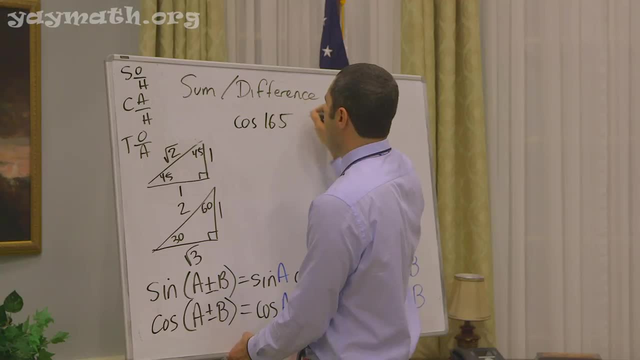 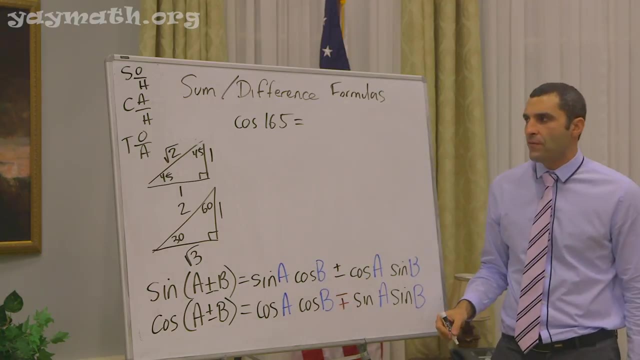 Cosine, Cosine, Cosine, Cosine, Cosine. Okay, Find them Inside. 165 are 30, 60, 90 and 45, 45, 90s, Keeping in mind that we could be in Quadrant II. 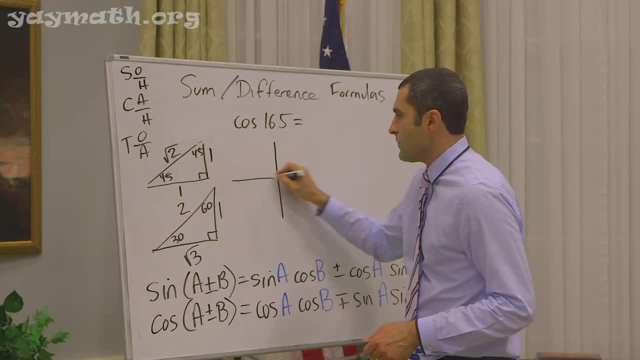 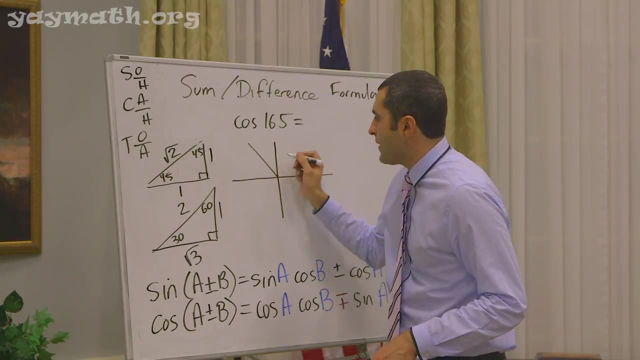 Don't think of just Yeah, We could be in Quadrant II. This is in Quadrant II, isn't it? Yeah, It makes more sense to be in Quadrant II And think it like you could do if I did 120,. 120 degrees is hovered over the top. 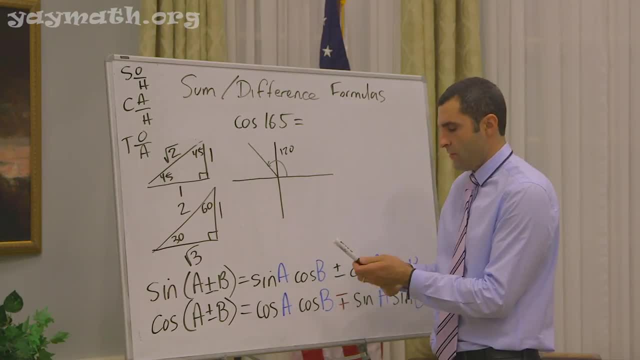 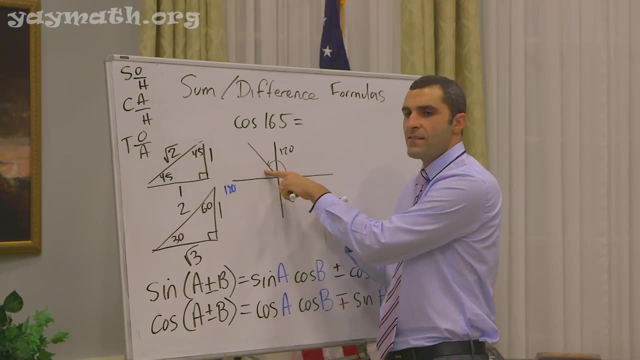 What is how many degrees in here? um 120 degrees in there, so what would it be in here? up to 180, 150, 60, oh, 60, 60, yeah, yeah, so you could say 120 and you're really talking about 30, 60, 90 in. 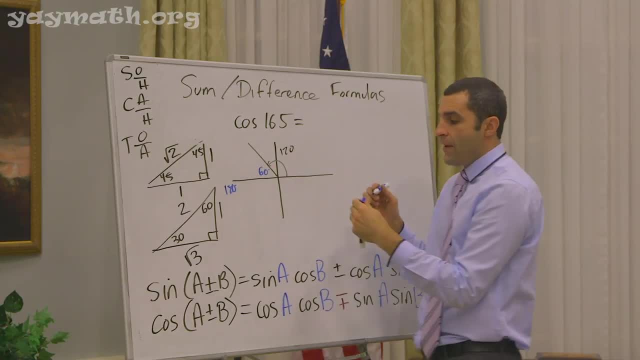 quadrant two. so you could say: 120 plus what? perhaps plus 60, 40, 45, oh 45. okay, 120 plus 45 makes 165. okay, that makes sense. and 120 is nothing more than a 30, 60, 90 in quadrant two. 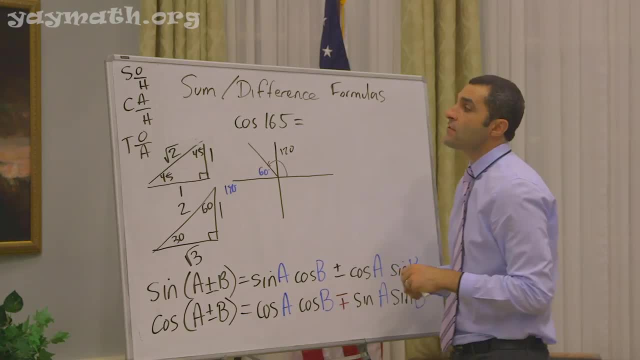 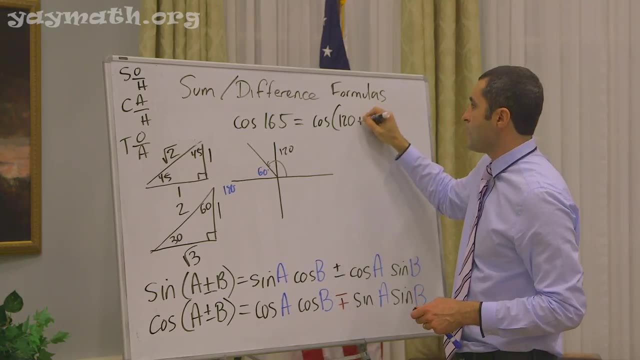 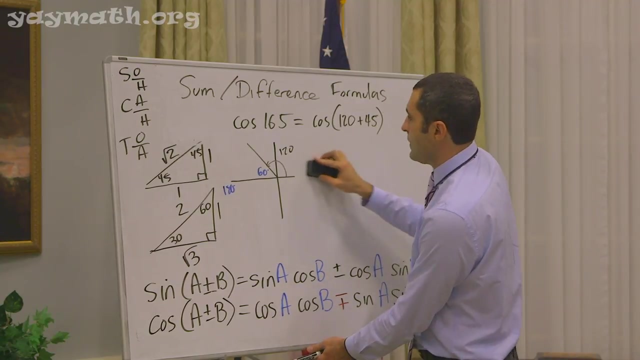 that's all it is, and we'll put this triangle in here. perfect, okay, so let's do. yeah, we'll split this into um cosine of 120 plus 45. okay, um, i'll leave this. actually, i'm gonna take it off and put it over here. i'll stack them. 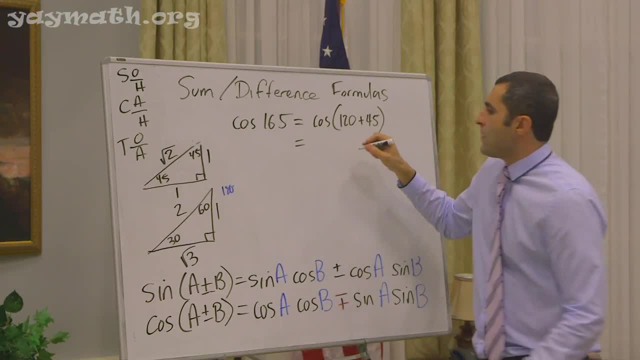 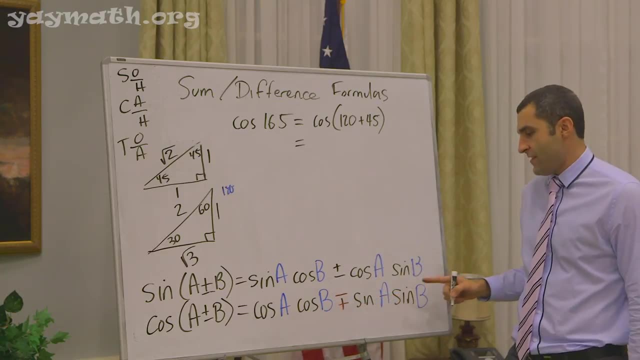 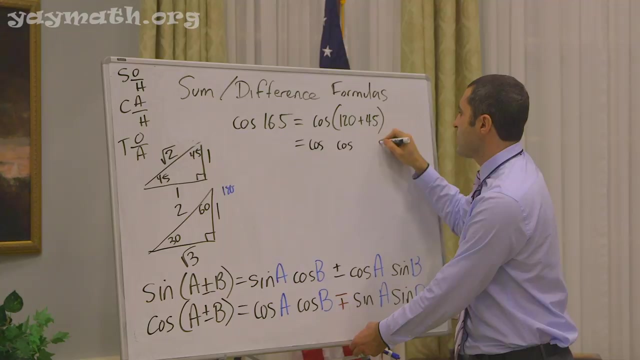 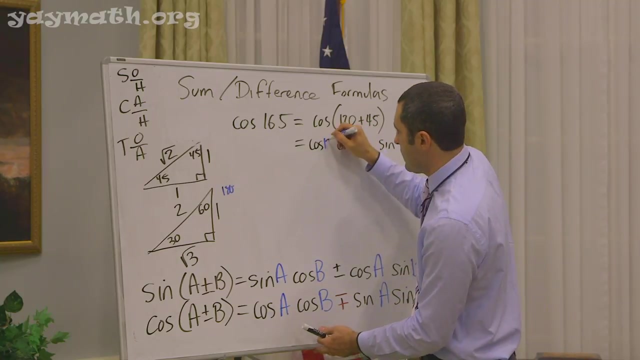 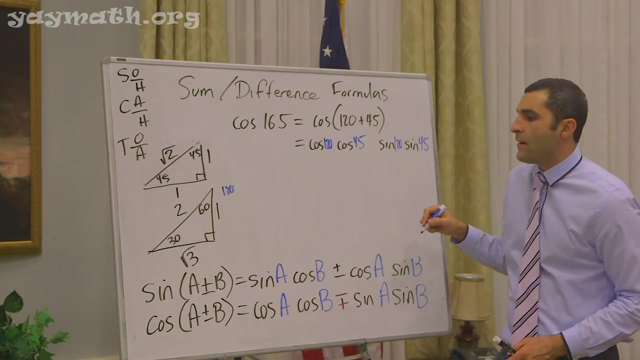 so let's split it up for cosine. and so we did sine, cosine, cosine sine. and there we go: cosine, cosine sine sine. now we can go straight to the numbers: cosine, cosine, sine sine. the numbers would be 120, 45, again and again. and now tell me what the sine would be: minus, minus, minus, plus, minus. oh, it's plus, here it. 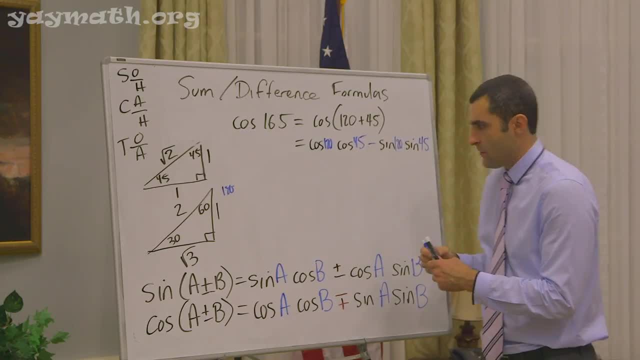 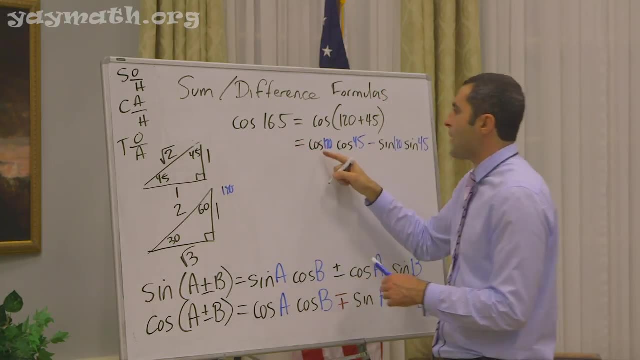 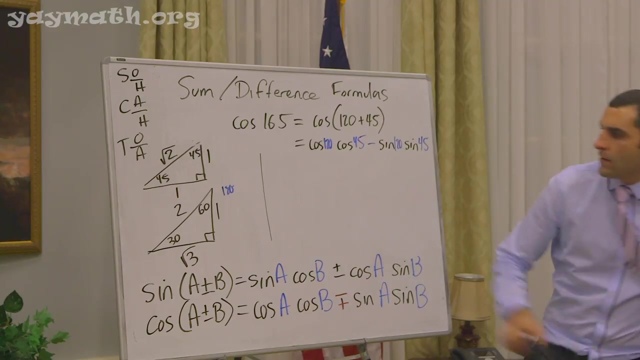 switches. well done, it switches. oh man, i love positive, i'm a positive person, me too. i'm such a positive person. i know me too. all right, let's do so now. we're talking about 120 and 45, so basically, in like the two, these two quadrants over here. try to use this well. 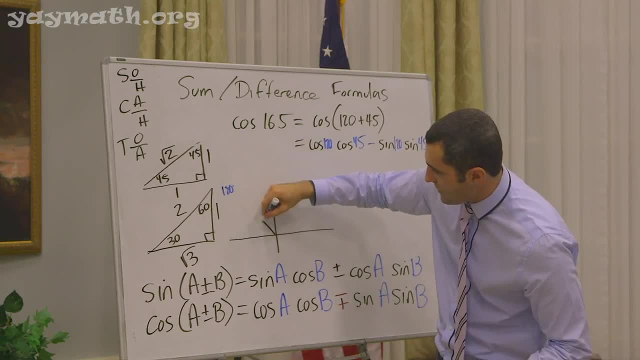 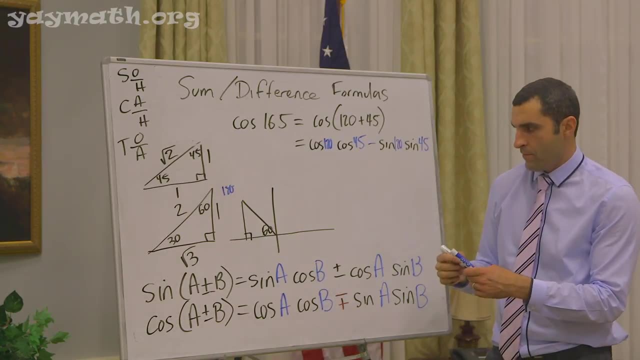 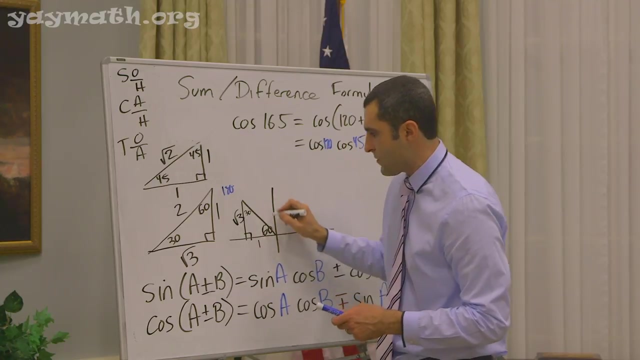 so let's do 120. 120 is a 30, 60, 90. yeah, over here, let's fill in this triangle. across from 60 is what uh is, wait, root three. good, well, across from 30 is one, one, hypotenuse is two. are any of these negative? 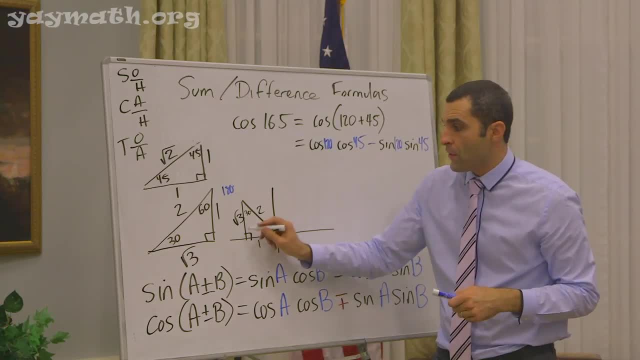 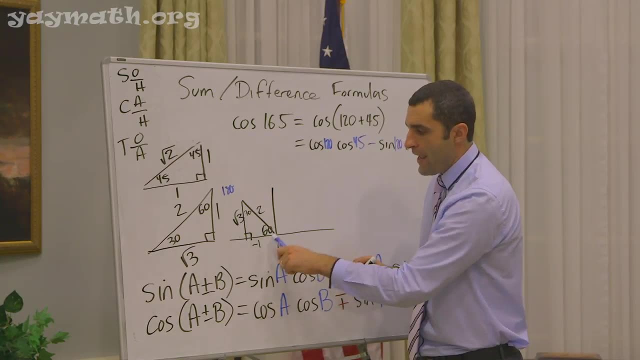 no, yes, yes, root three. root three is going up and negative, oh, negative, just negative. one negative one is hypotenuse, ever negative, no, no, so yeah, root three is going up, for y is negative, moving left. so that would be good. so there's your 120. let's also do 45s in quadrant one. 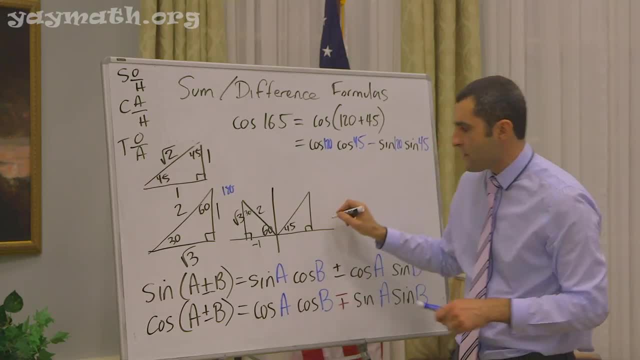 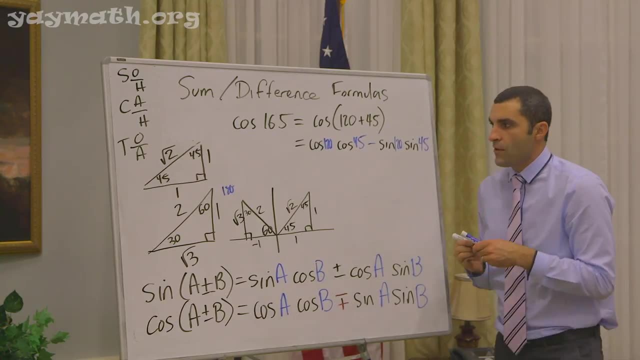 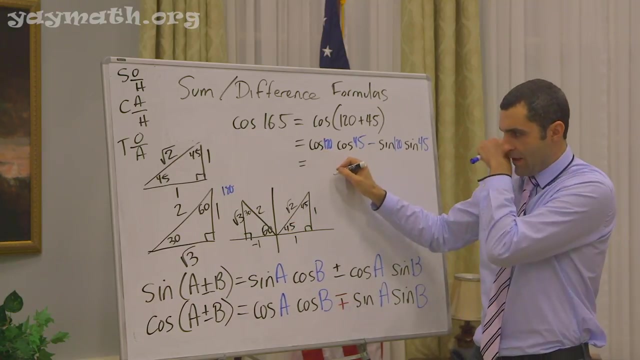 is anything negative in quadrant one? no, correct size for 45, 45, 90, hook it up right. one, one, one, one, two, two, very nice. now let's go ahead and fill it in. cosine of 120. here we are. what do we get? um, oh, 60, you can, yes, cosine of this 60. exactly what is the cosine of the 60? it's, it's negative. 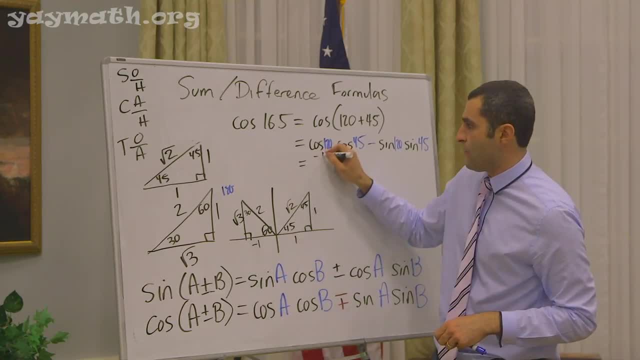 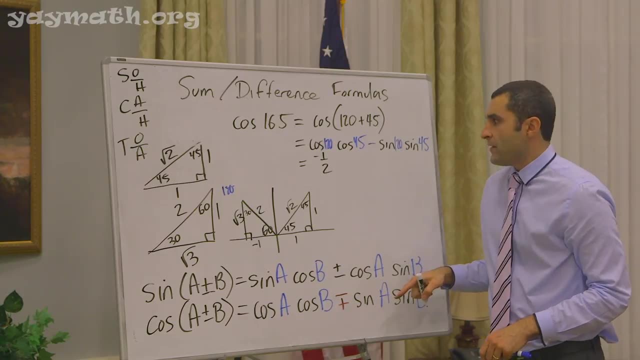 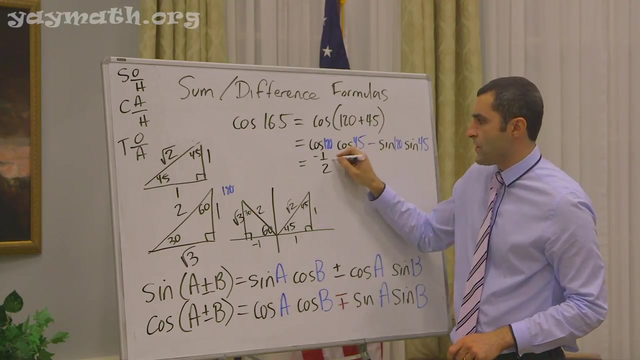 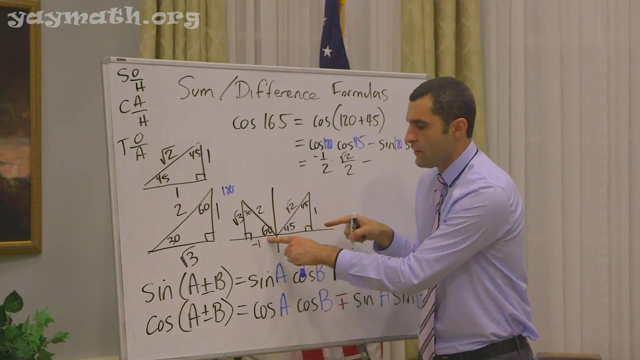 one over two, excellent, negative. one over two, cosine 45. here we are, you're doing great, oh great. one piece at a time, uh, one over one, and a two, one over two, yep, which is two root, two over two root, two over two, very good, minus sine 120. here we are, sine 120, uh, it's gonna be. 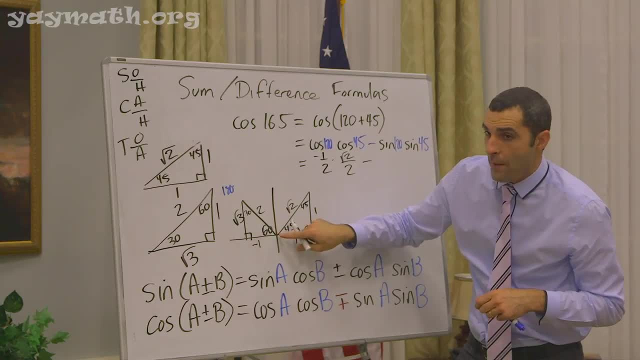 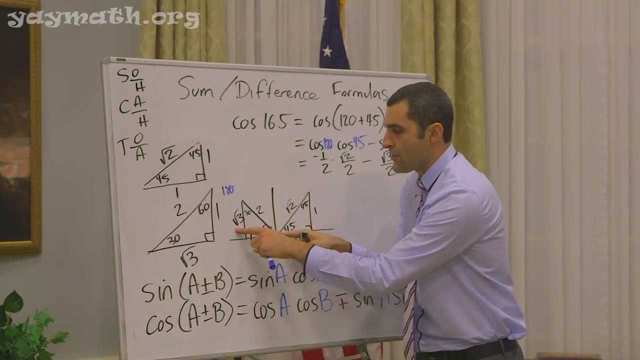 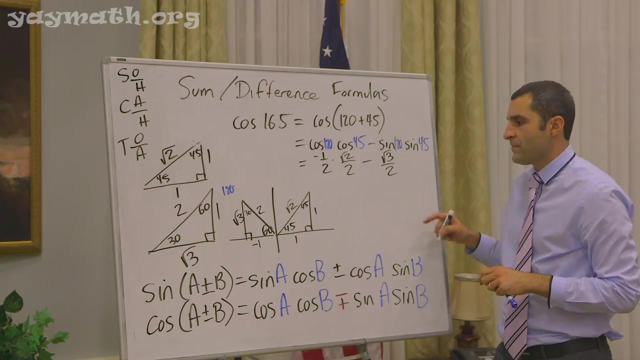 um, it's two, uh, negative one root three. oh yeah, we're like over two. root three over two. opposite over hypotenuse. it's correct, sine is opposite over hypotenuse. root three over two, and now we're back to 45, sine 45.. it's gonna be, uh, one over two. so two, oh yeah, yeah, all right, okay, and now we get. 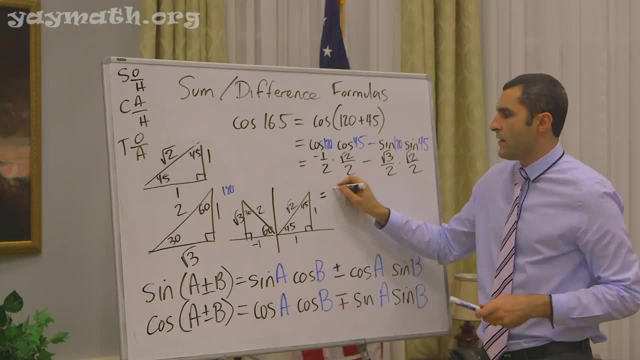 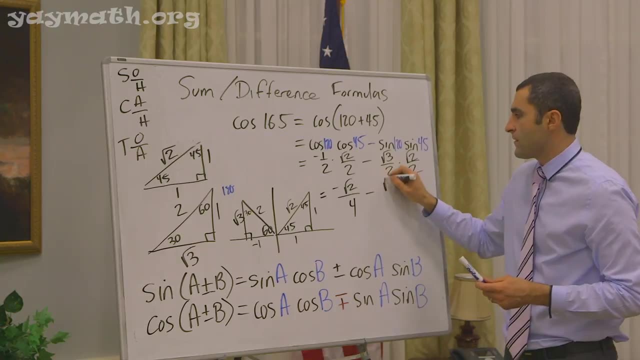 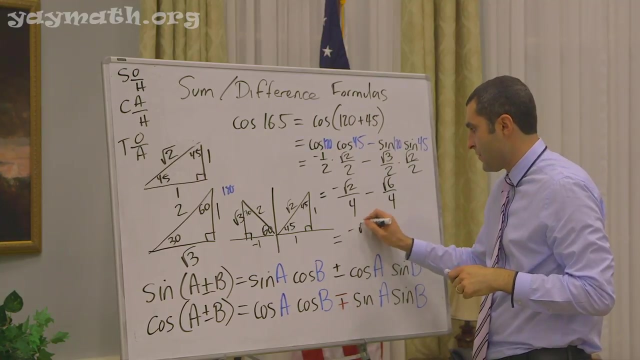 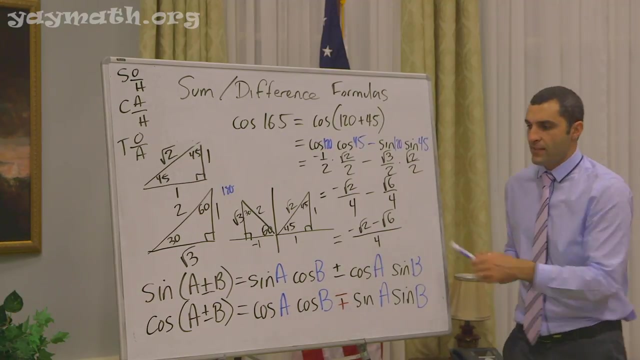 upstairs. try again. over four, Bravo. all minus root. six over four: yeah, combines to one fraction, yep, and then it's just negative root two minus six. six over four, all over four, very nice. and again, we can check this on the calculator. but this is the answer by checking. you put in 165 in there, because I'm 165. 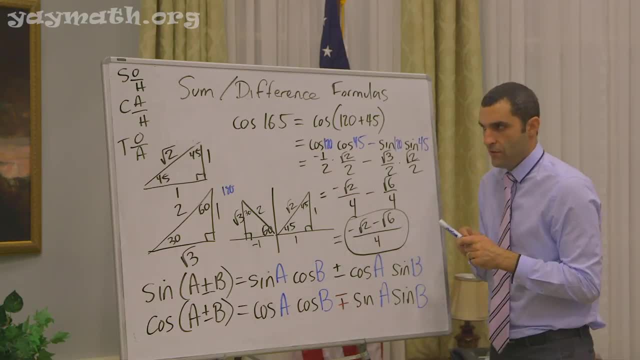 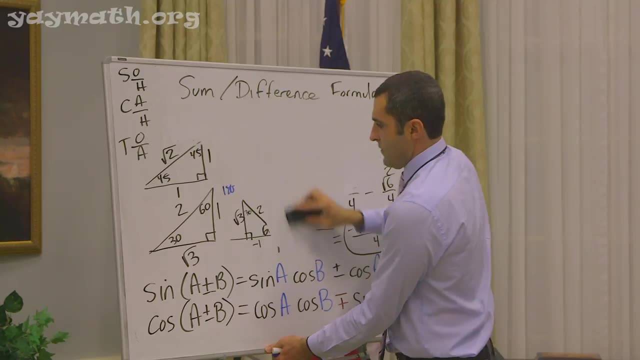 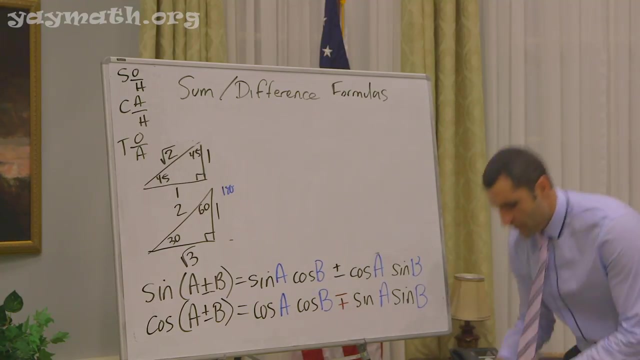 This ratio? Okay, Cosine 165, is this crazy ratio? Perfect, That is great, man, It's really cool. Woo, All right, Keep it going, All right, Ooh, Okay, We have a different genre of problem. 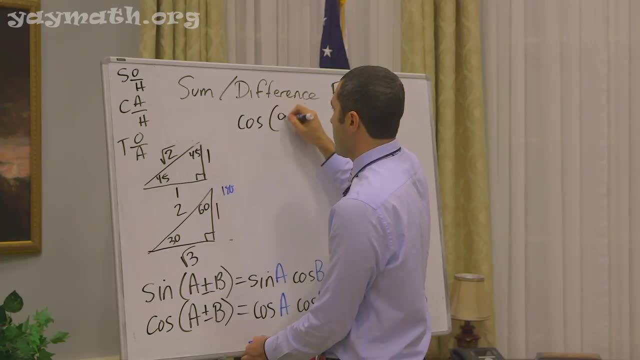 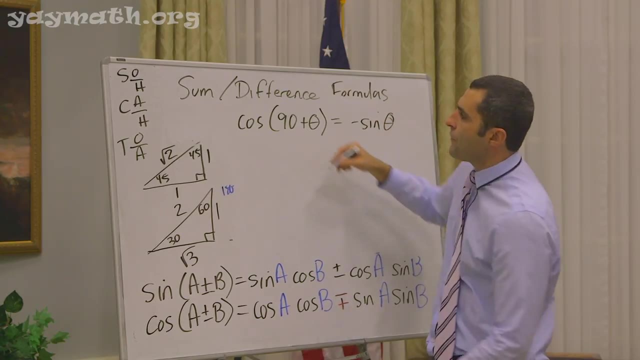 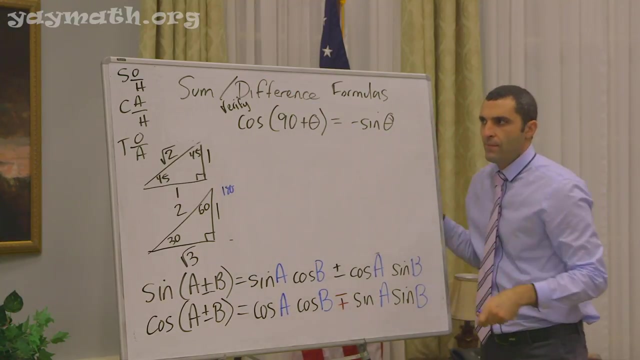 Fear not the genre Boys. Cosine of, let's say, 90 plus theta equals negative sine. So this is a verify problem. You have to verify that the left is the same as the right, So it becomes cosine 90?. 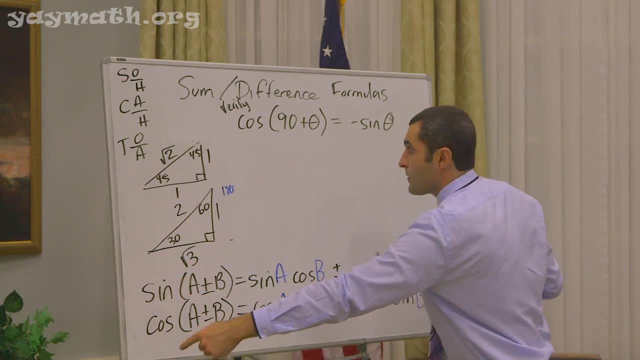 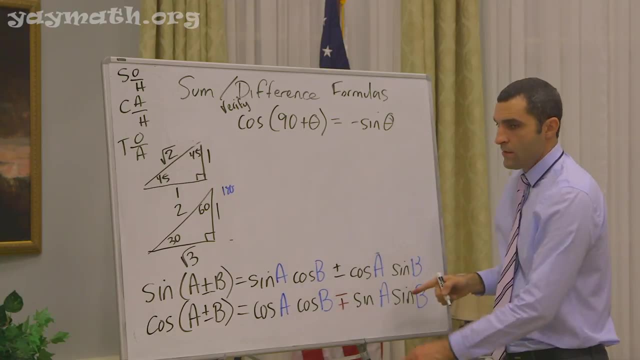 Shall we do split. Which one? is it The first one or the second? Well, it's the 90.. It's the first one. Sorry, the second one, Cosine of A plus B. There it is, Yeah. 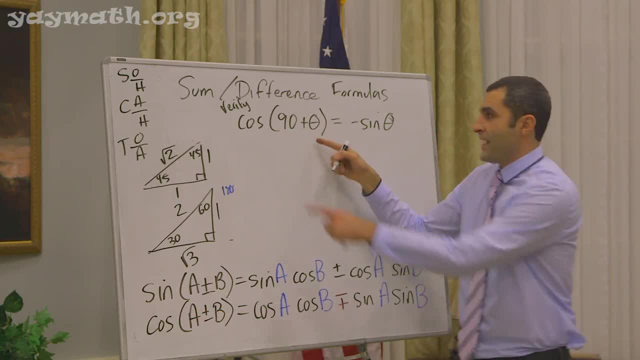 So we're going to expand this. Yeah, And the exact one here is cosine, cosine sine sine. So we'll go: cosine of A plus B. Cosine of A plus B, Yeah, Cosine of A plus B, Yeah. 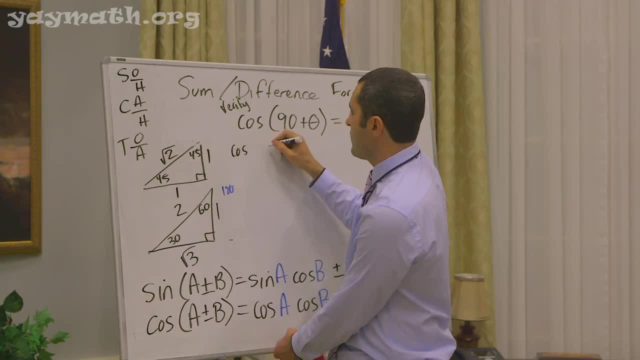 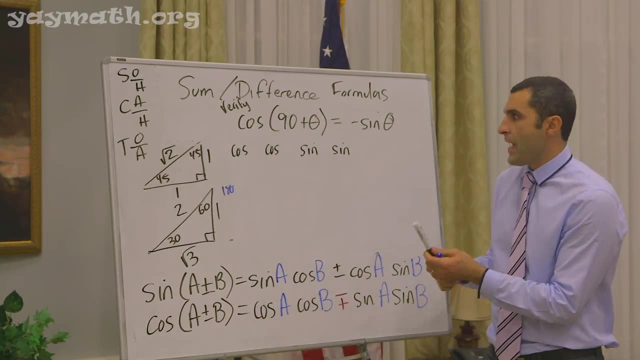 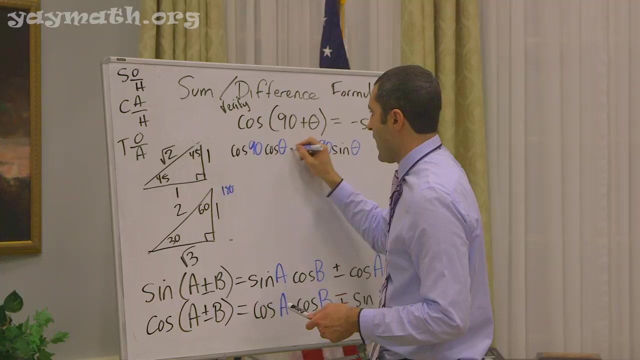 Cosine of A plus B. Cosine of A plus B. Cosine of A plus B. Cosine, and it's minus. yes, it is sine sine. and put in our angles: 90 theta, 90 theta minus, and it's minus correct. yes, all right, let's see what we get. so we 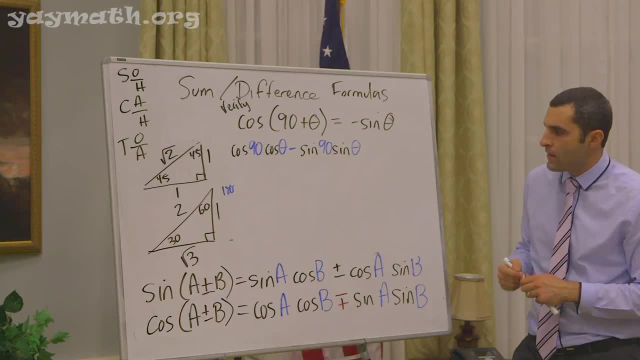 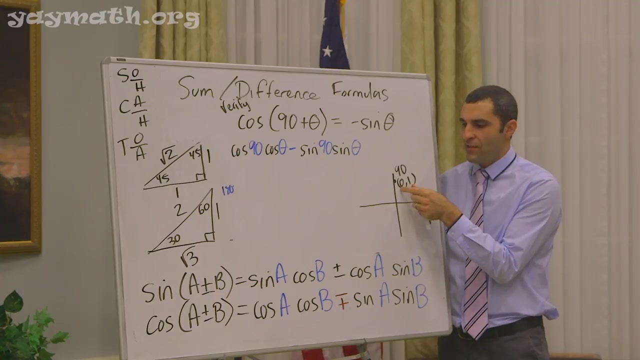 have cosine 90 unit circle time. let's put our unit circle up: 90. where's 90 90 is? I can the second. what's the point? the point, yes, what is cosine of 90, 90, 0, 0? what is sine of 90, 1, 1, sine of 90, 0, sine of 91? good, what's the sine? cosine of 90. 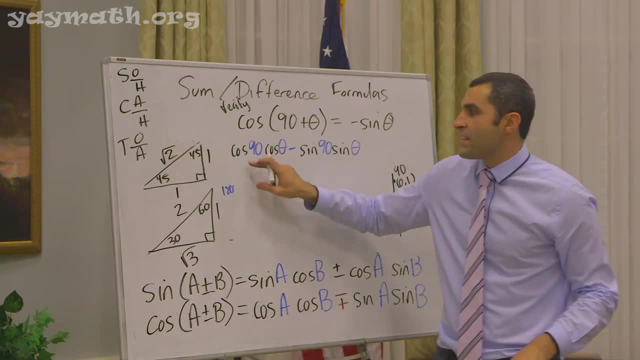 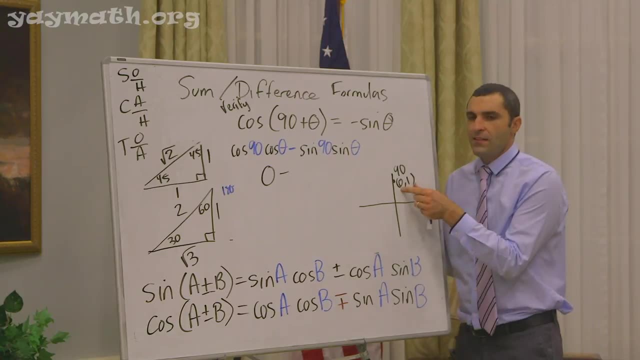 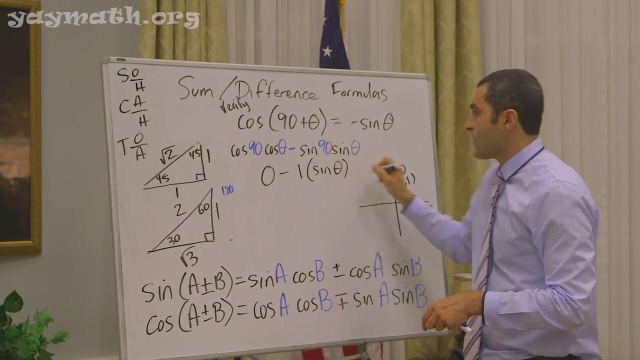 then 0 Bravo, 0, 0 times cosine theta is 0 minus. now we're back at 90, this one. so it's 90, which is negative. ninety right, negative, no, not negative 90, you know what you mean. what's sine of 90? 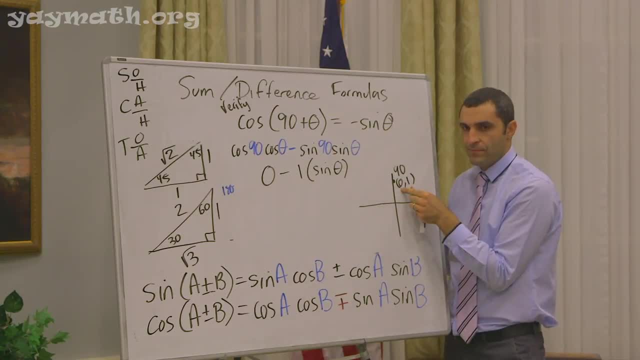 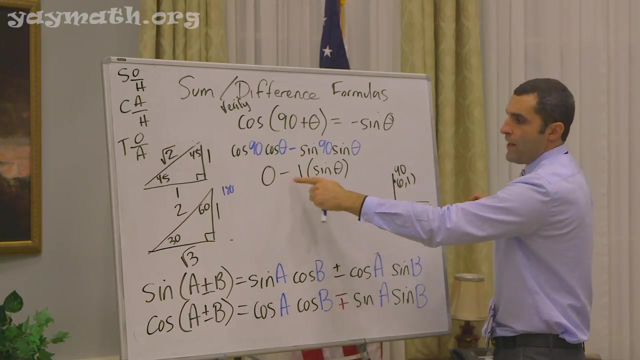 sine of 90, is it 1 times sine theta? uh-huh, okay, this sine of 90 became 1 sine theta. came down: what is 0 minus 1 times sine theta? what is 1 negative one? next, you go ahead. so it's just negative sign data and there's your verification. 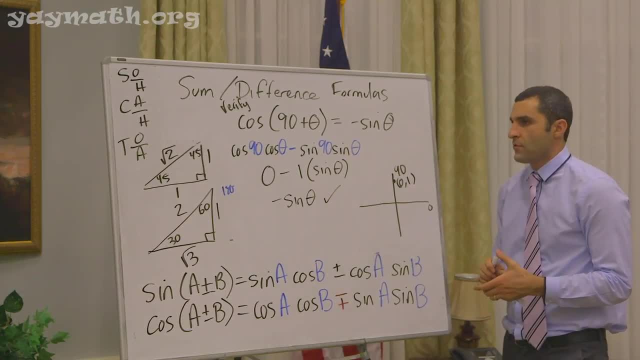 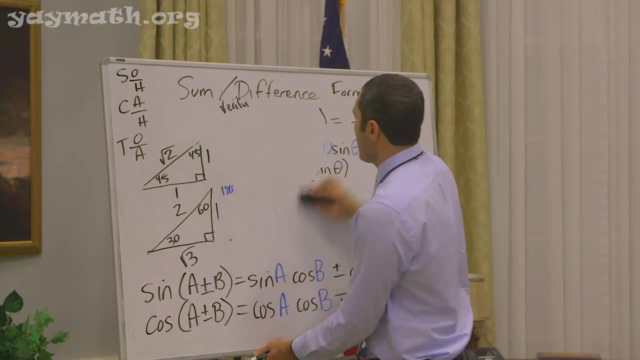 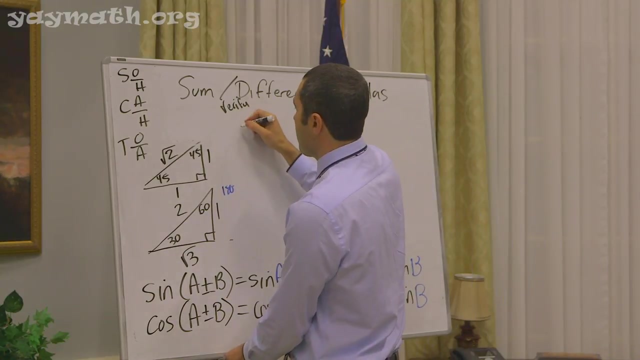 wow, all right, you want to try another one? sure, let's do it. another one will help. like that, solidify, we'll forget. should we get in some tan action? yeah, we're gonna get. that's the second. that's the second last one. then we have tan. so this one is verify. sign of 30 plus data. 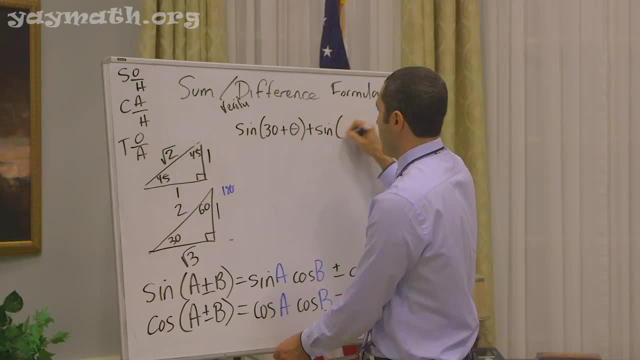 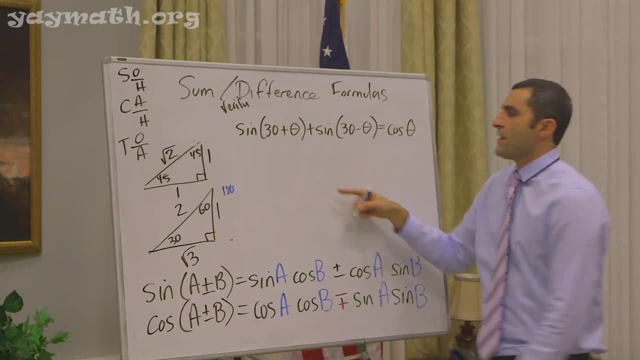 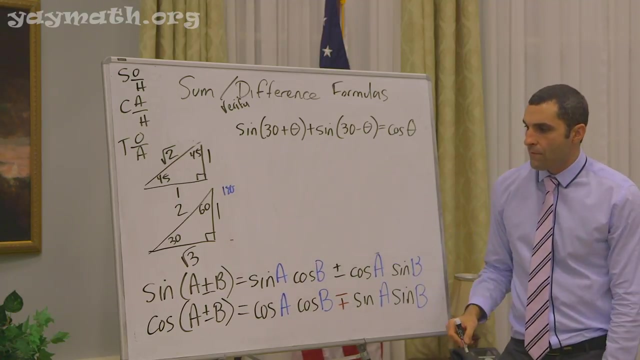 plus sine of 30 minus data equals cosine, isn't that? it's just? it's crazy to me that all this noise results in cosine data. so we're going to verify: split it's the. is it first or second? second, first, first, that's what i meant. i was looking at sine and i said second. i believe you. 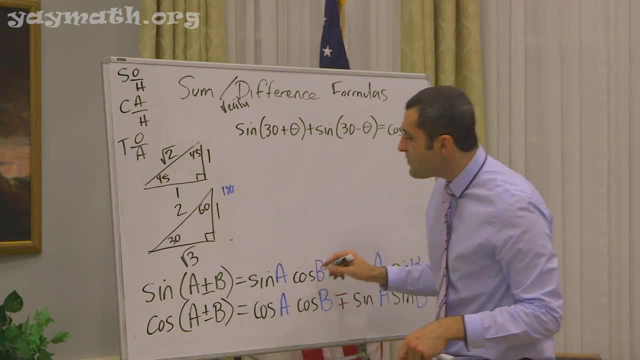 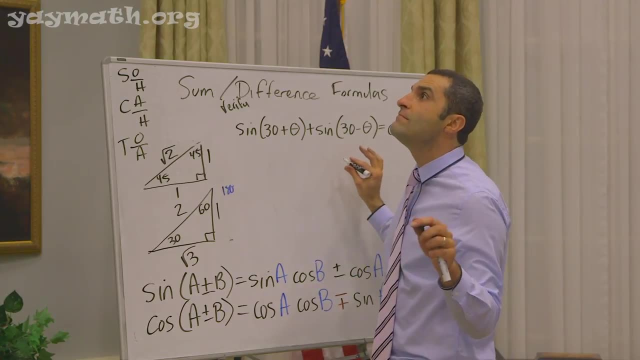 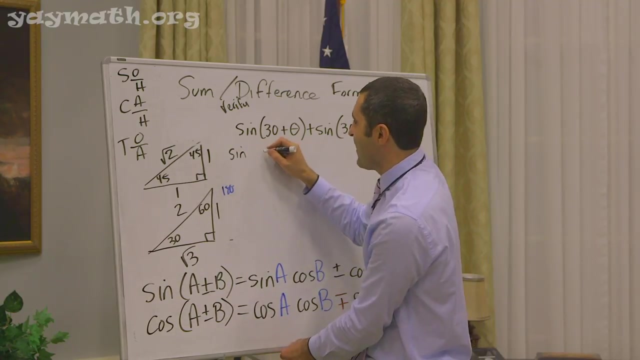 i believe you let's do it so we have sine cosine, cosine, sine, sine. that's that- harmonies at some point. yeah, we got at the end of the video, let's try harmonies, okay. oh, with with tree, that'll be fine. sine cosine, cosine, sine. why don't we just handle? 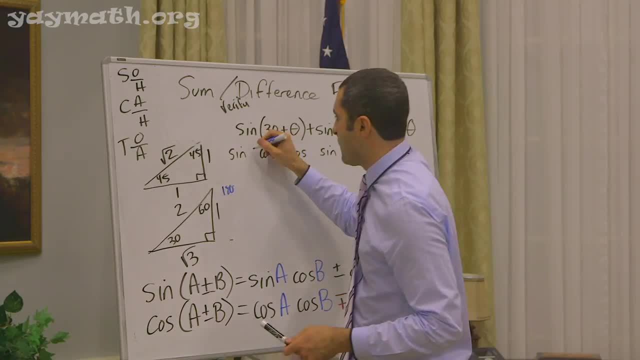 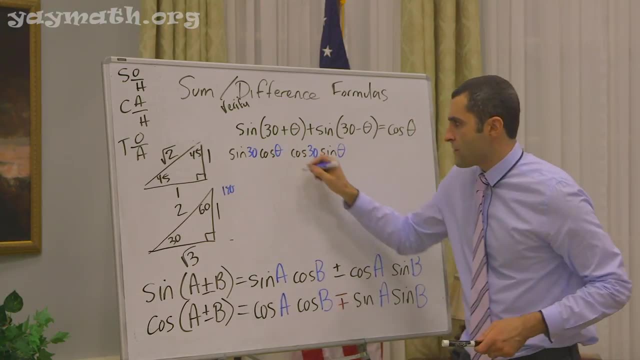 this one first, sine 30. yeah, so we put our angles in 30 theta, 30 theta. yeah, you want to tell me if it's plus or minus. tell me it's plus plus. yeah, good, would you like to do this first or would you like to get this one? 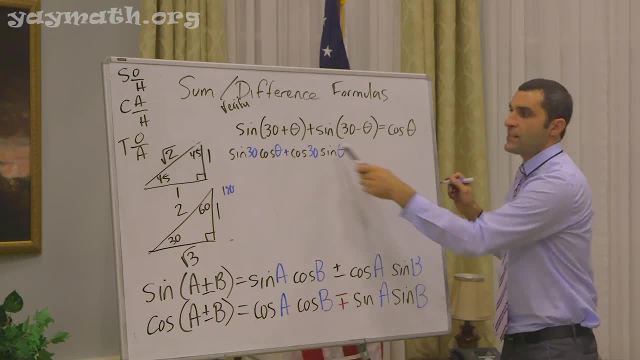 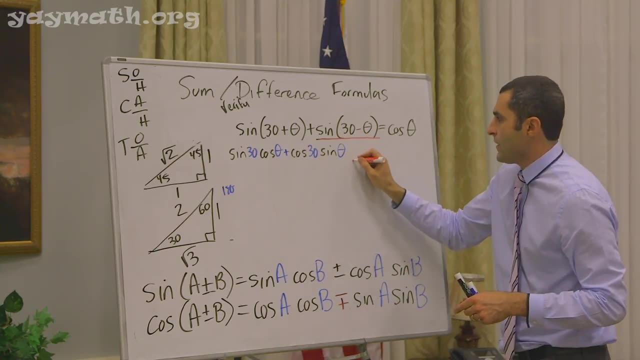 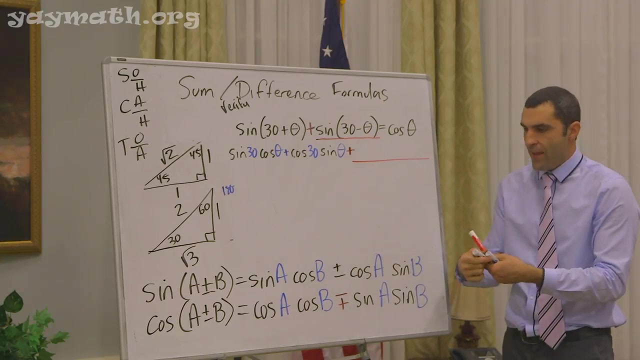 you expand it and then do it all. yeah, we can expand it. let's expand the second one, sure? so i'll underline that in red. this thing is now going to be expanded over here. right, we have a plus. yeah, this is the plus, this is the plus space. all right, so expand the sine sine, cosine, cosine, sine, and write it. 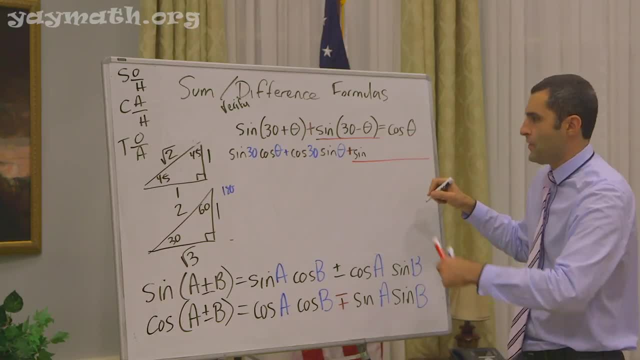 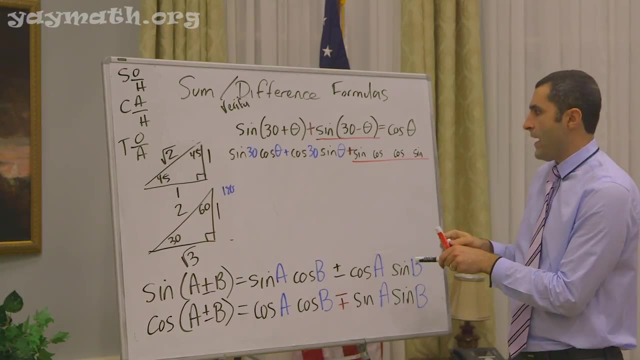 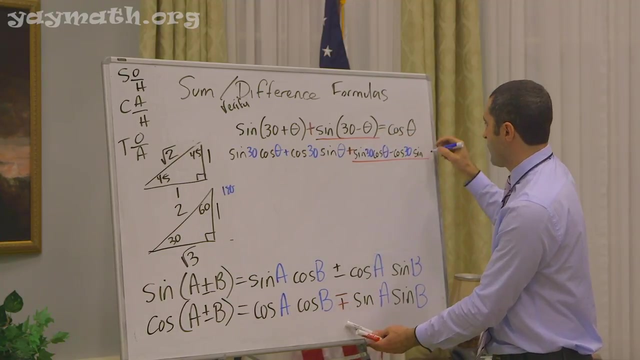 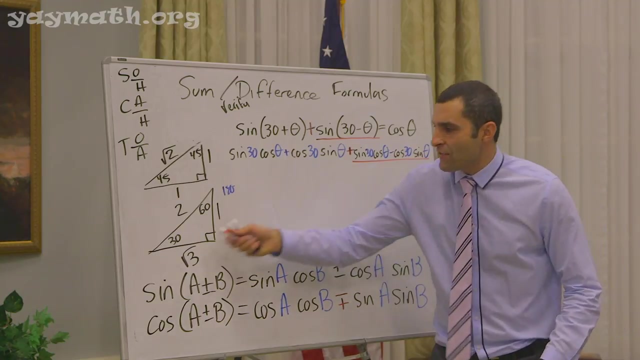 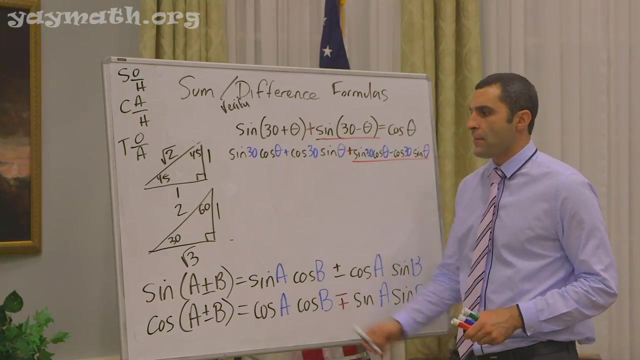 is it the same? and then the same thing. it's the same thing, except it's minus good, plus sine 30. sigma, right, putting in the angles, you're right. bam, oh, all right, all right, now we're going to go piece by piece. peace, okay, uh, sine 30, it's right here. oh wow, we can just use this: 30, 60, 90, of course it is 36, gently. 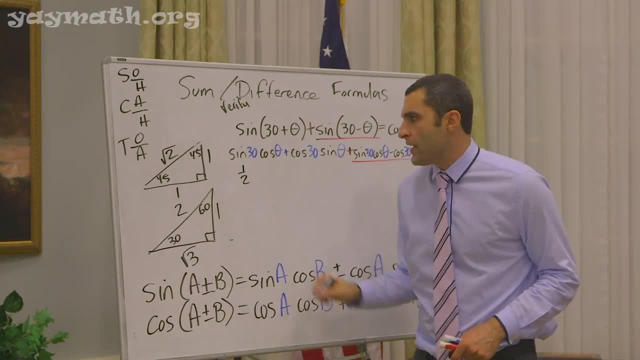 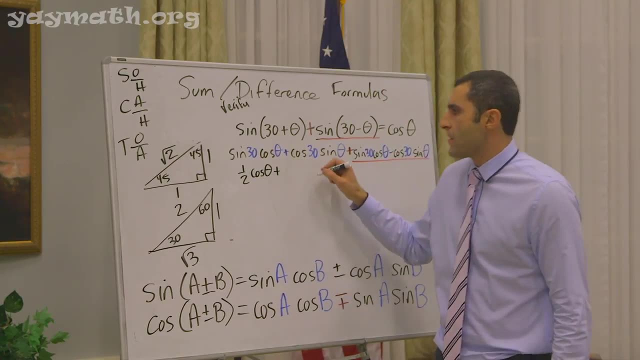 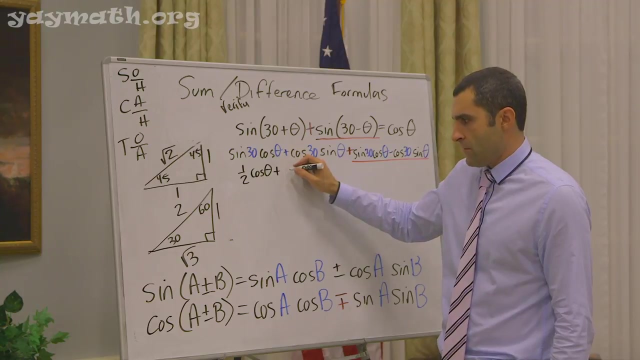 one over two cosine of theta. we don't know what theta is, so we just write the cosine theta. okay, one half cosine theta, that's all of us plus cosine of 30 right here, which is: this is no wait, cosine of 30 is is a root. 3 over 2. Jason over. 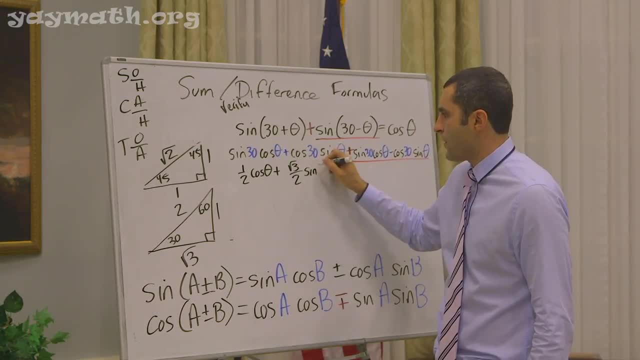 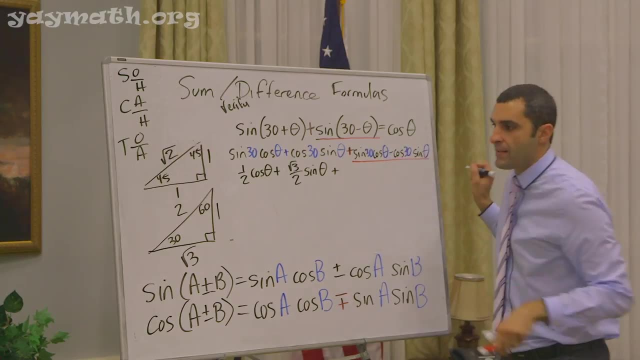 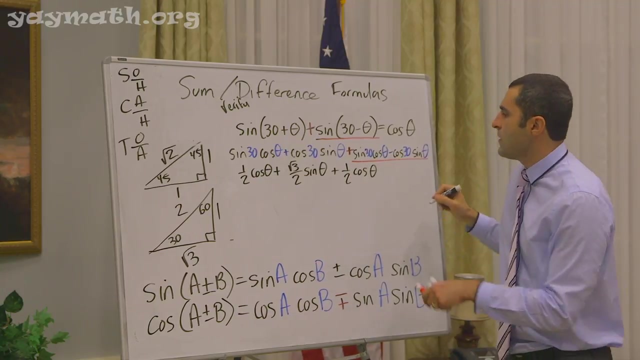 hypotenuse root 3 over 2. very good times sine theta. we don't know what it is. plus, here we are at sine 30, cosine of the angle. so back to sine 30, one half cosine 30. that's right, let's just give me cosine the angle, thank you, thank you. 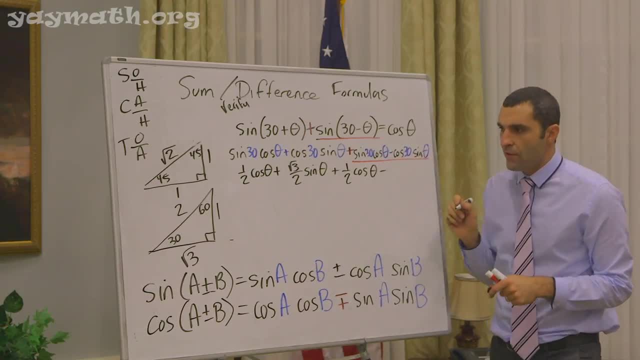 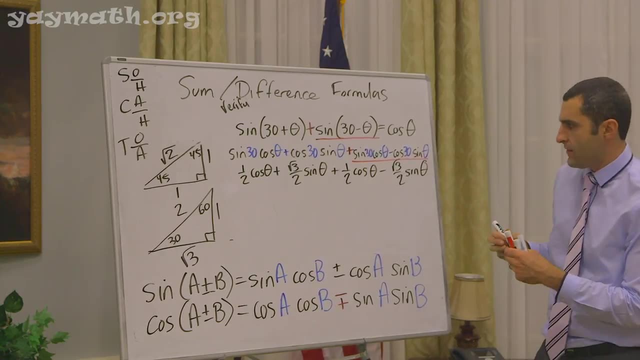 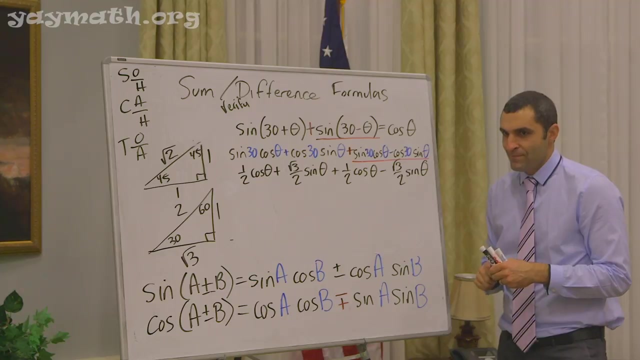 minus cosine 30, which we did already. 3 over 2. root 3 over 2 times sine of the angle. all right, what do you see? we all it simplifies into cosine theta. it does, because one half of that plus one half of that becomes one. but then the root 3 over 2, sine theta minus root 3 over 2. 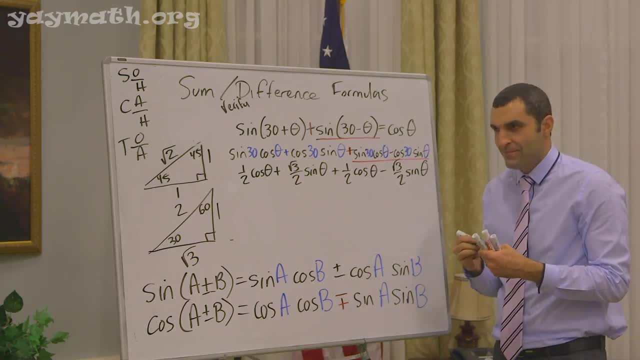 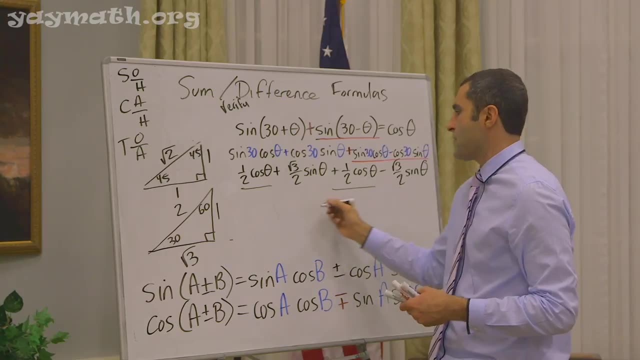 sine theta. yeah, it cancels out. so then, but then two halves make all yes, and have we verified then, yeah, we have verified. so you're saying one half plus one half cosine is cosine theta. let's be even more explicit. we go bam and bam and we 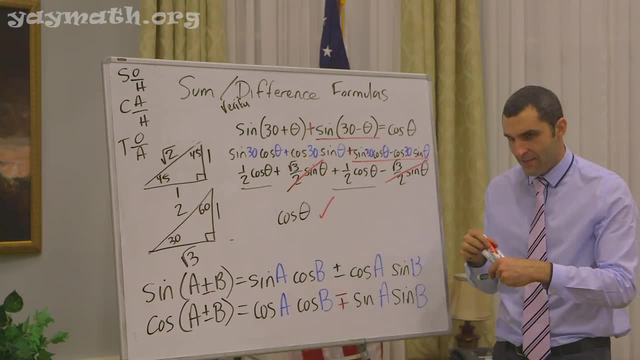 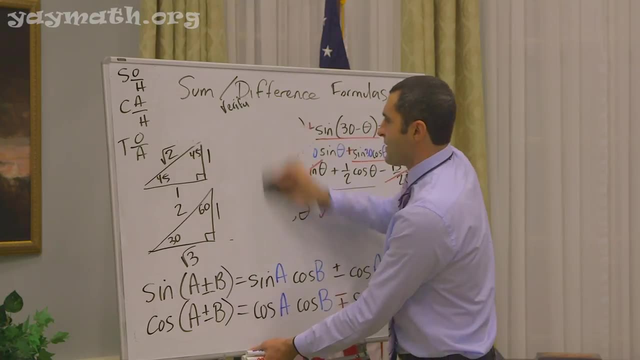 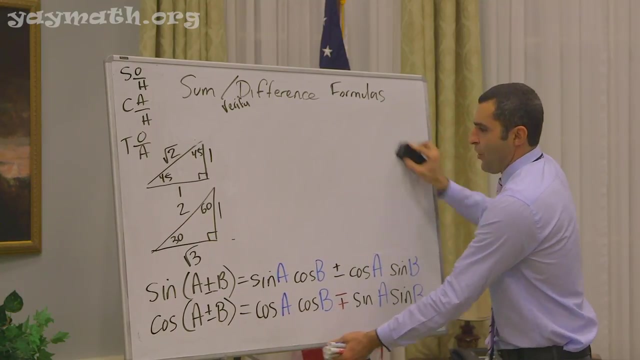 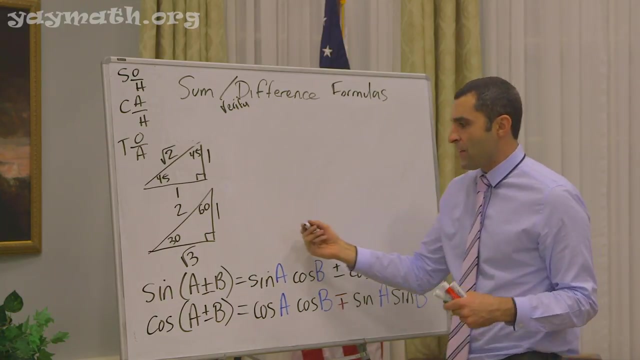 got a verification. this is done. look at that. okay, let's do one more involving tangent. whereas my dad say would say back in the day, tangent time for my dad, tangent okay, time okay, touch, all right. so again, I don't expect you to memorize this formula, I have to keep looking at it. over there there is a huge derivation of the. 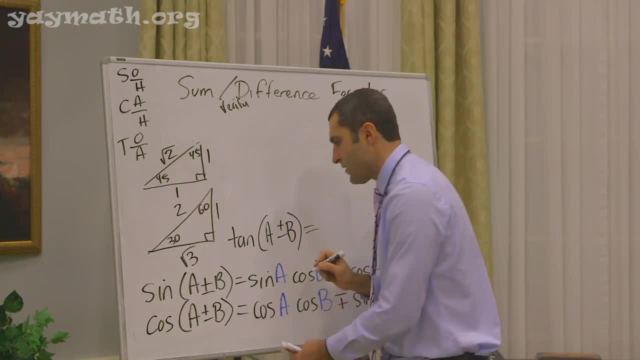 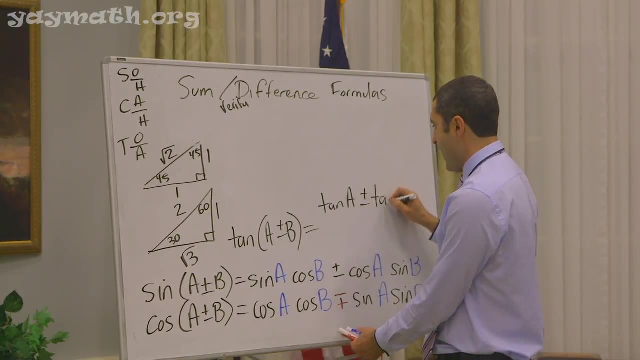 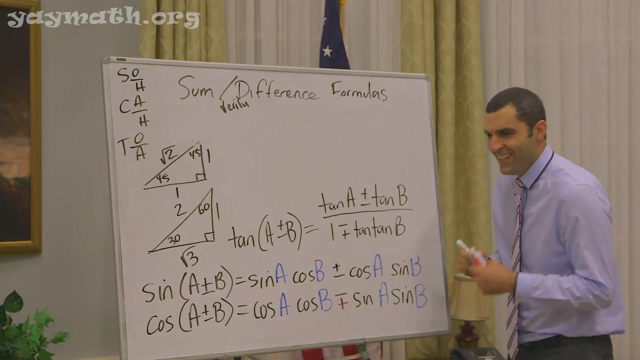 but don't worry about it. you know, if, as long as you can work with it same format here, I don't have a song, if you want to be the first in history to make a song, you may. so what is? oh, you want to do it to the same tune? let's do it. okay, there it is 10, 10, 1, 10, 10 maybe. 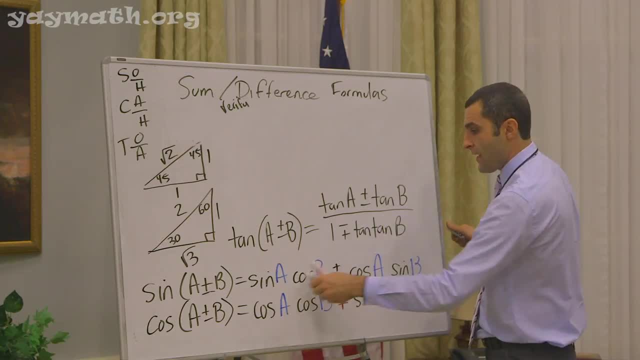 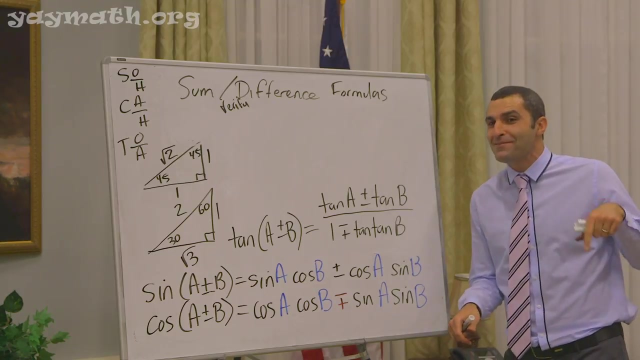 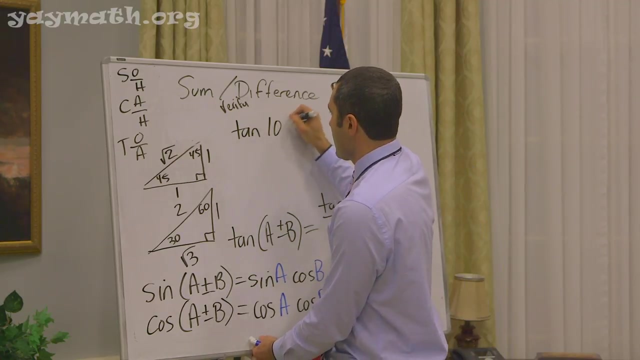 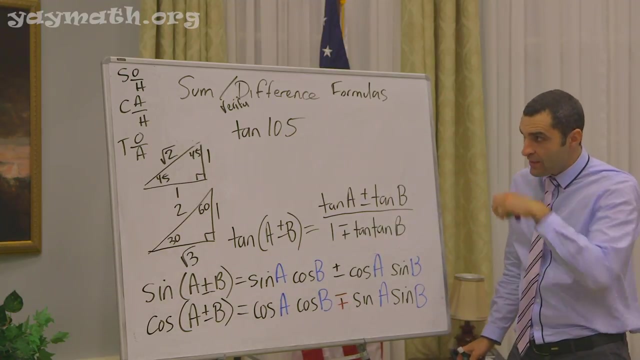 it can be the third one, right? so if sine cosine, sine cosine, cosine, sine cosine, cosine, sine sine, all right, last one we'll do is 10, 105. all right, find the two angles hiding inside that. are these? okay, so it's for, it's one of. 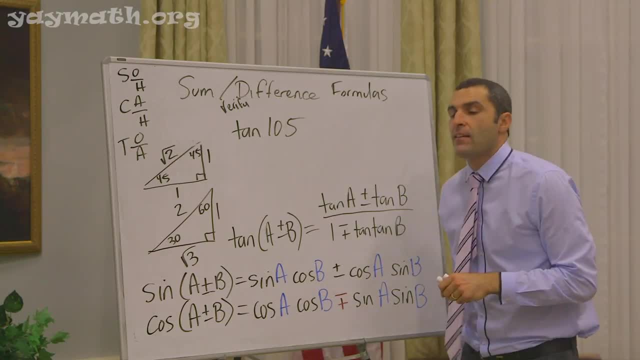 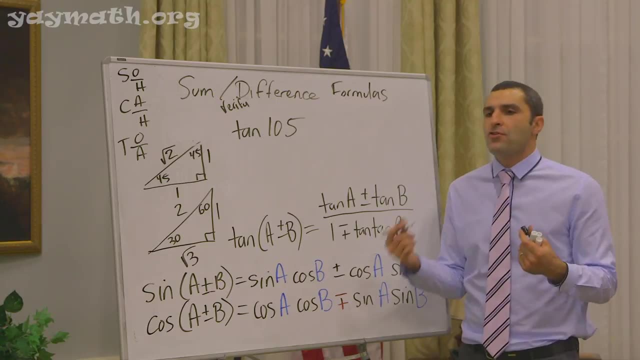 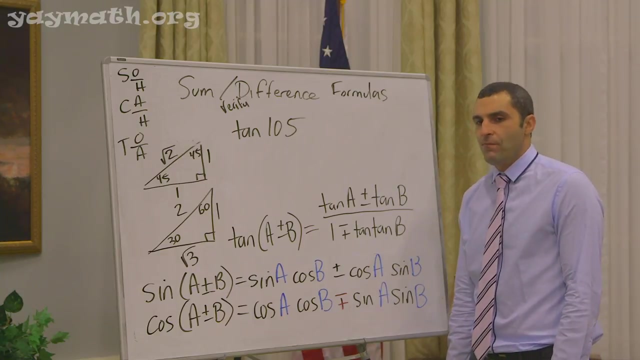 the 45s or 3690. yeah, oh okay, and or because it's in this, it's in the first quadrant. no, it's in the second quadrant. yes, but we don't know. we don't have a 105 triangle. yeah, so we need triangle like values inside here. that works. there are two that you can add: 45 plus. 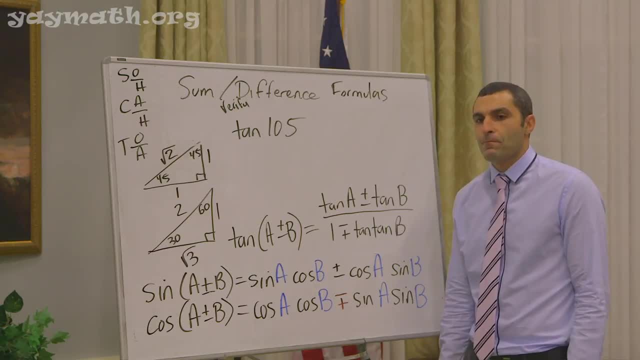 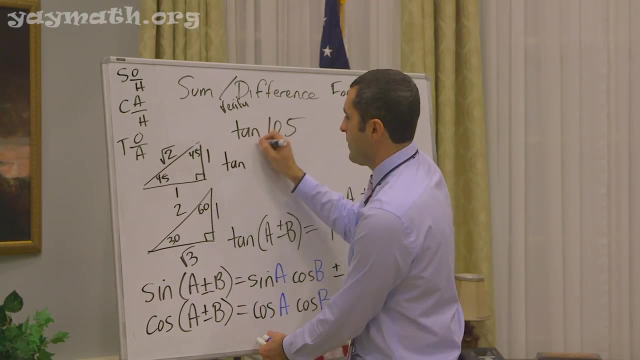 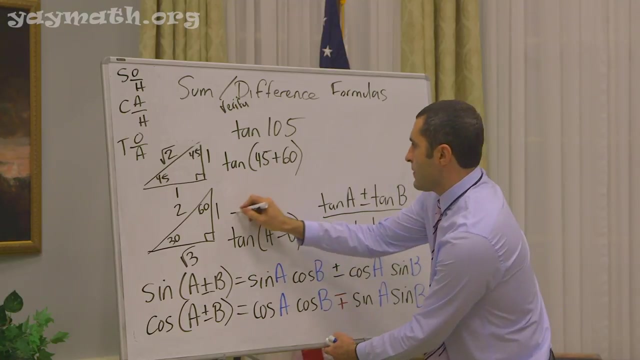 plus 160 plus 60. yeah, 45 plus 60. okay, let's do it. so this is really 10, 45 plus 60. you'll notice, check it out. this is: let's make this. this is plus or minus. this is plus or minus minus this. 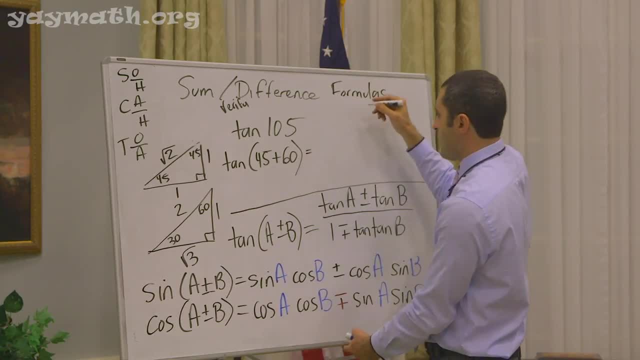 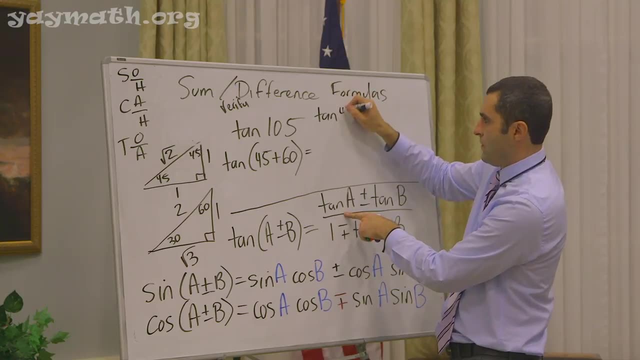 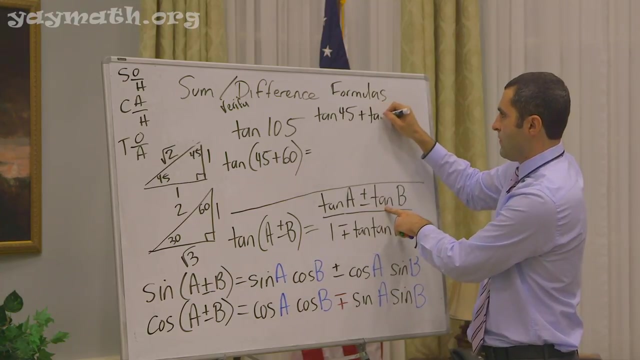 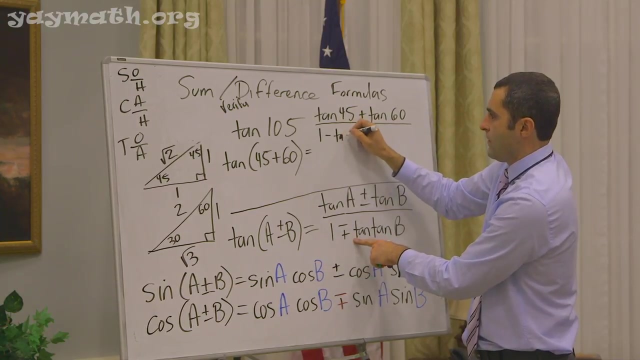 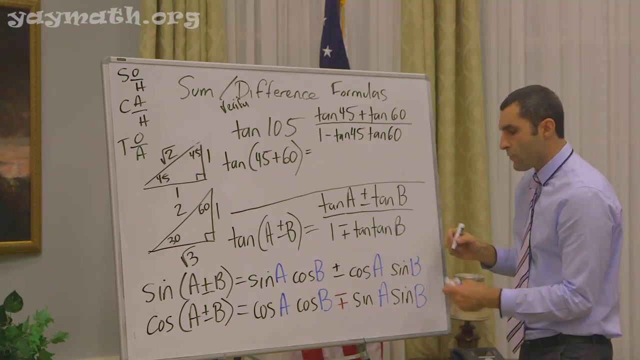 is minus plus. yes, all right, we got this. will go straight to the numbers. so this is 10 of what. it's 10 of 45. what sign? uh, plus plus. that matches tan 60. all over one minus one minus one minus tan tan 60.. oh, 10, 40. oh, we forgot the 10 a what? oh yeah, that's a 10 a in the formula. oh good, thank you. 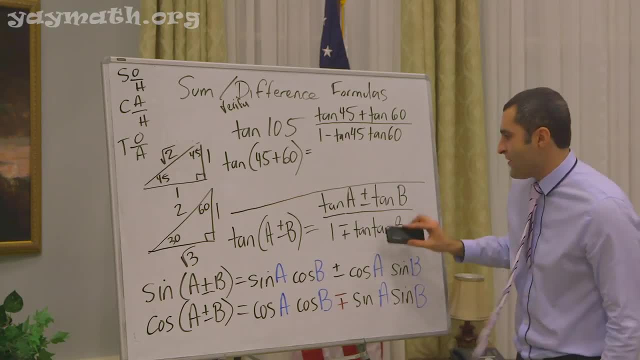 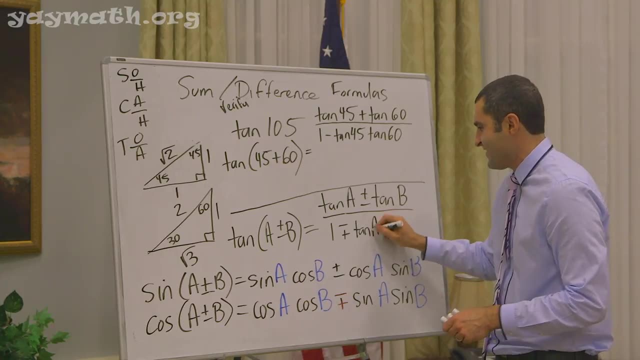 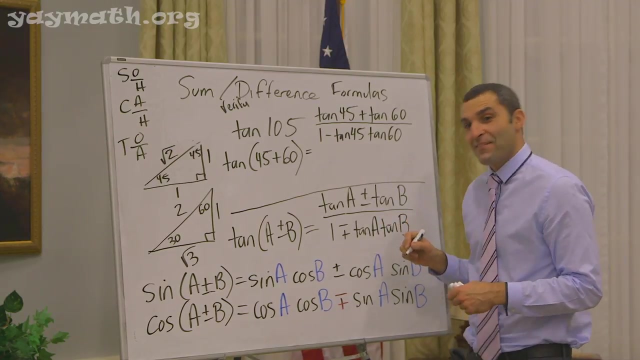 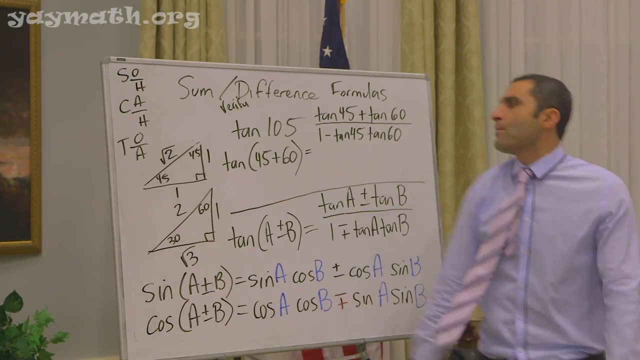 oh, i was too caught up with the song, we got too excited. yeah, ten, 10, one, 10, 10.. there it is. ten, 10, one ti 10. put it on itunes, but on spotify, patent pending or copyright pending. uh, all right, 10, 45, boom Лун 10, it's opposite over. 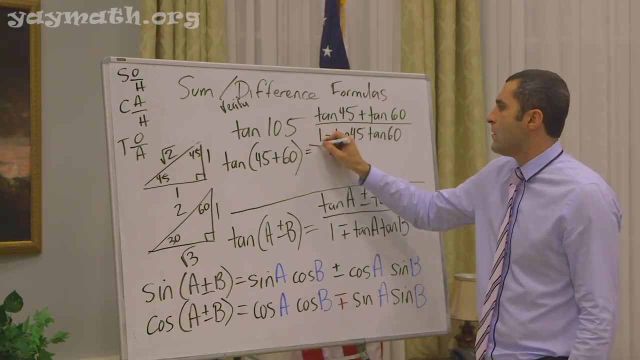 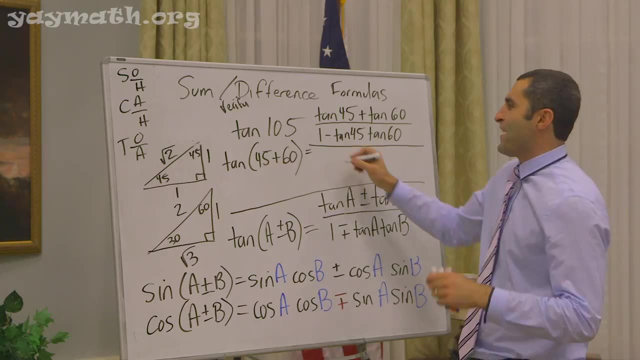 adjacent, which means it's one over one. it's not, oh, it's one over one. yes, you got. oh, oh, uh, it's not, Uh-uh, It's not One of you decide, So it's one One plus tan 60.. Tan 60, which is here. 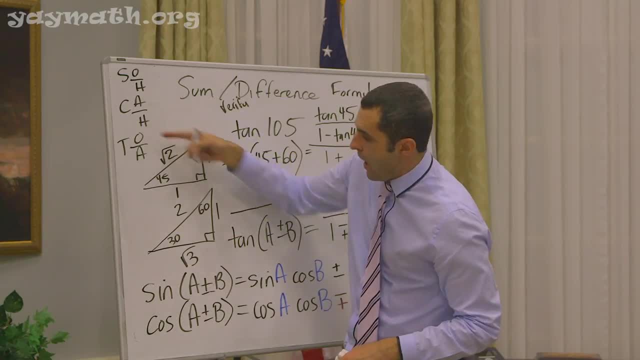 Oh, here it is, Here's 60. So tangent is Opposite. Opposite. Root 3, 1. Over adjacent, So it's just root 3.. Root 3,: very good, It's root 3.. 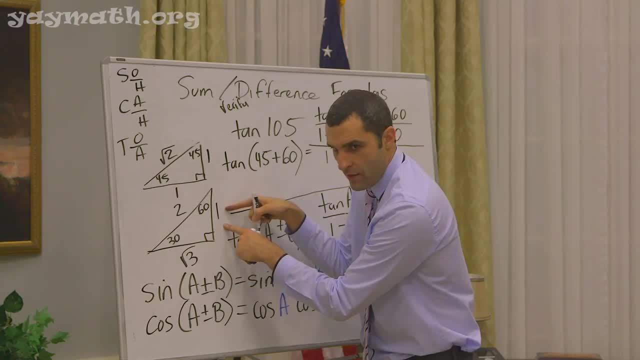 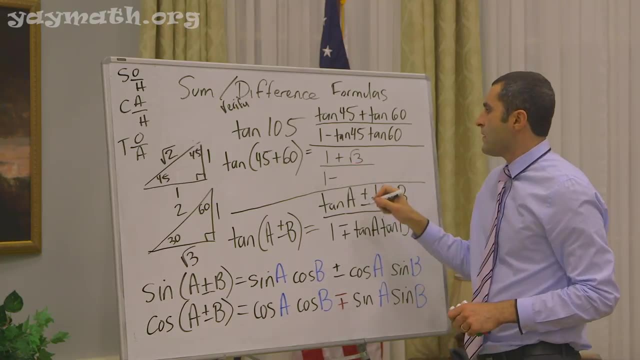 You see that Opposite over adjacent. I see Okay, All over, 1.. 1. Minus, Minus, 1 plus root 3.. Yeah, So 1 times root 3, right? Yeah, so it's just root 3.. 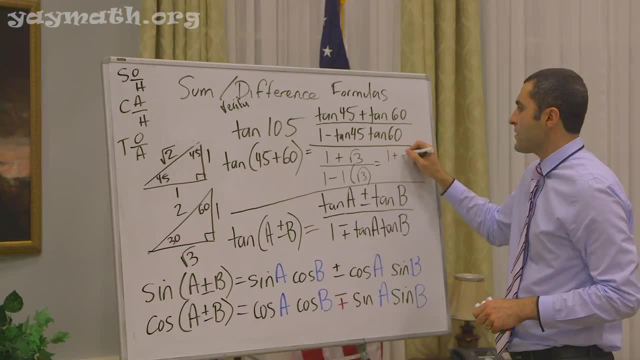 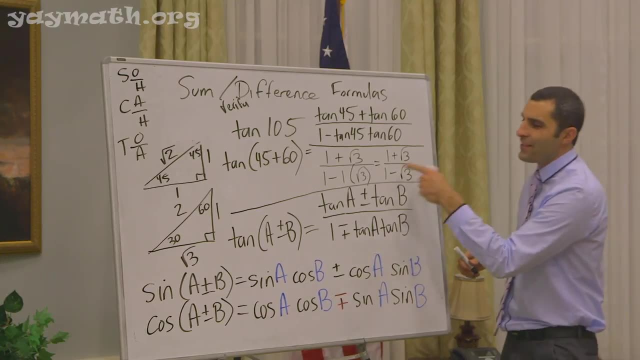 So, yeah, it's just root 3.. So it's 1 plus root 3.. 1 plus root 3 over 1 minus root 3.. Wow, You see that Now here's the issue: We can't leave radicals downstairs. 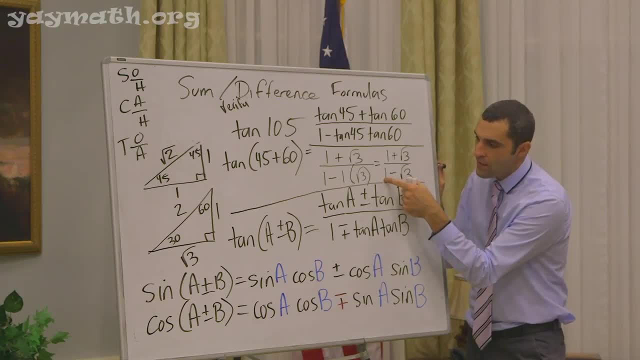 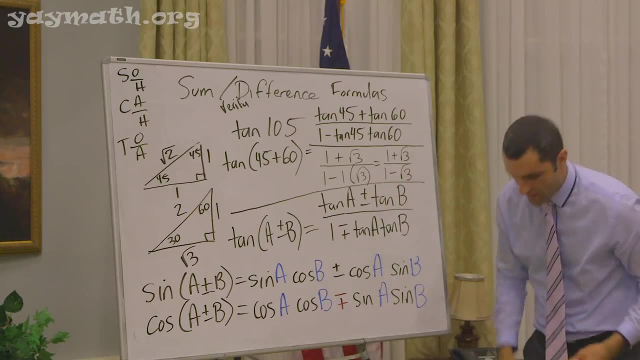 So we have to multiply top and bottom by the evil twin of this. It's called the conjugate, But the evil twin of this is 1 plus root 3.. Okay, we're going to do that. now. We're going to multiply top and bottom. 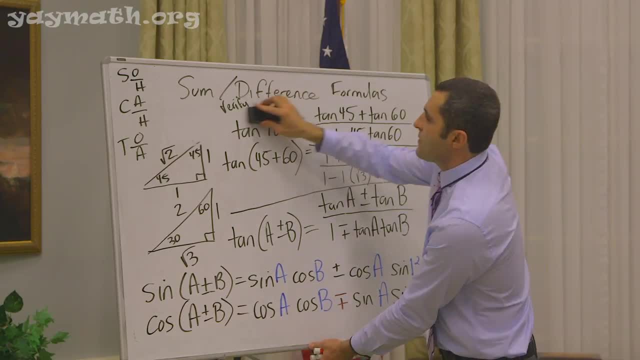 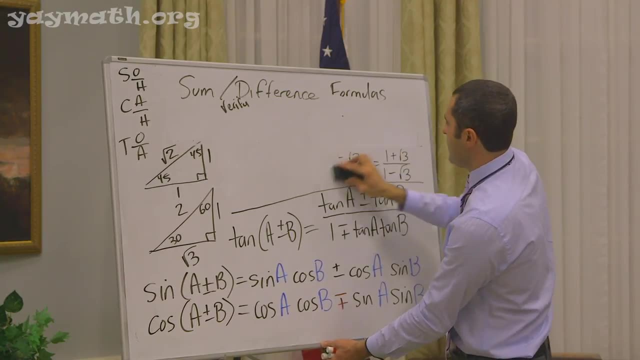 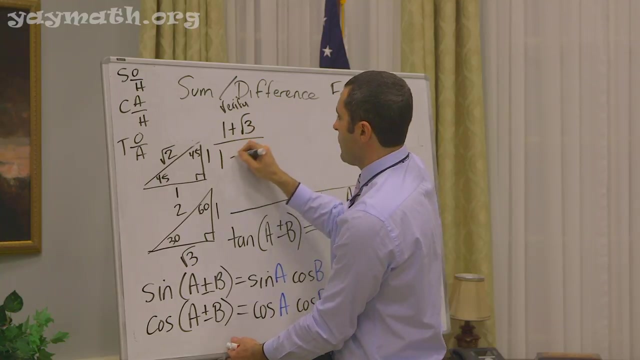 1 plus root 3.. You'll see It's going to be okay, So let's take this off. Okay, We did all these. Leave that where we left it here. Okay, So 1 plus root 3.. 1 minus root 3.. 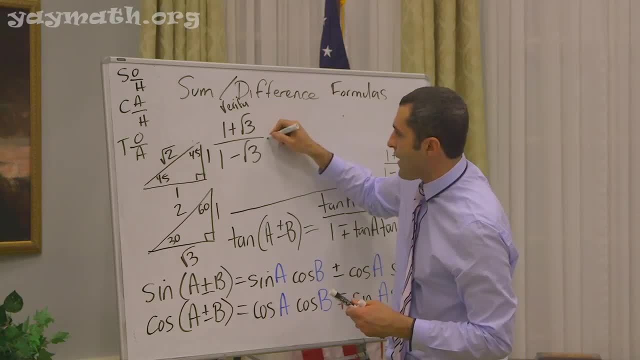 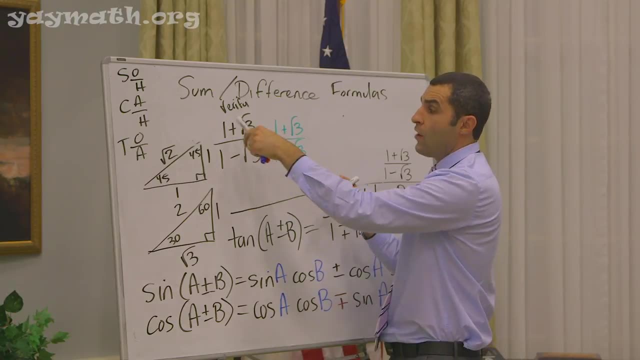 Multiply top and bottom by the only thing we can to cancel the radical downstairs. So is it 1 plus 3 over 1 minus 3?? Oh, you mean? Oh, this is the answer so far without being wrong. Okay, Okay. 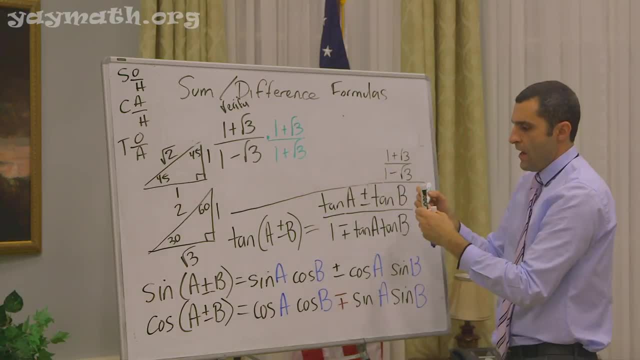 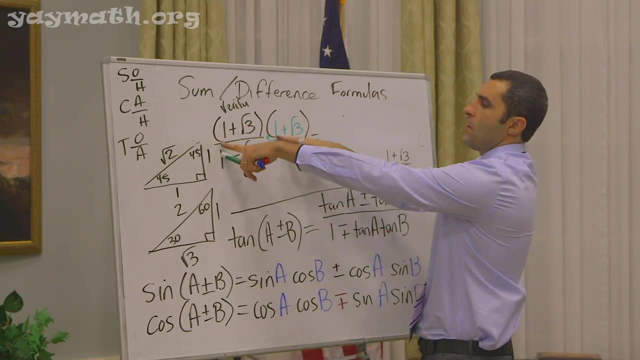 Okay, Okay, Okay, Okay, Okay. Let me simplify. Yeah, Yeah, So this is where we were, And now let's FOIL the top. Oh, we have to FOIL it, FOIL the top. Yeah, Equals 1 times 1 is: 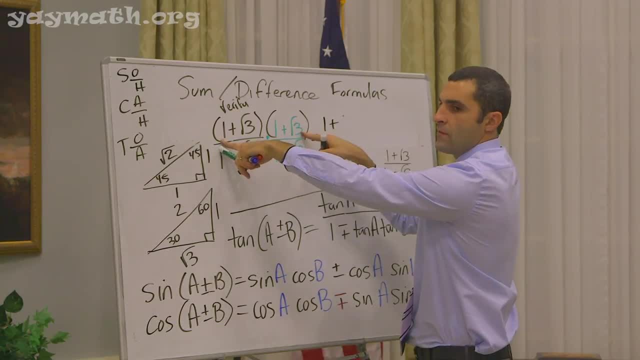 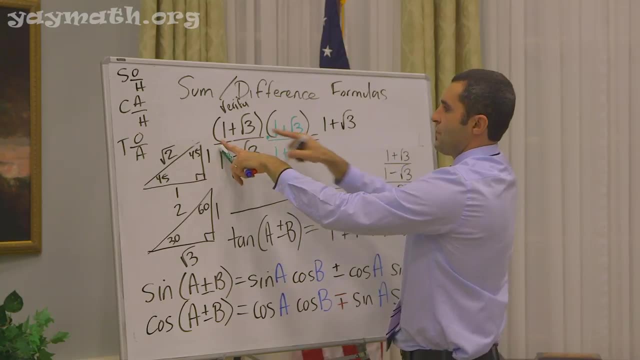 1. 1 plus. Oh, sorry, I can't see. So, Oh, it's, It's, It's Root 3. Root 3. That's first, Yeah, Outer Inner Root 3.. 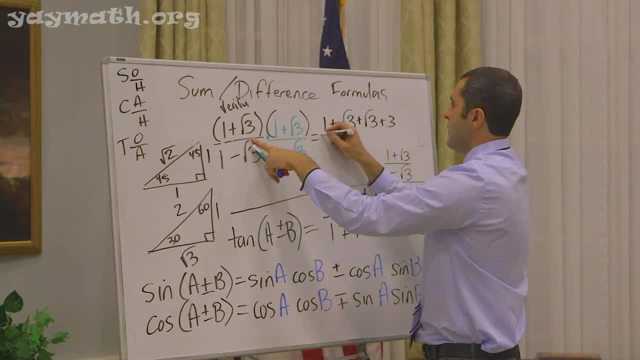 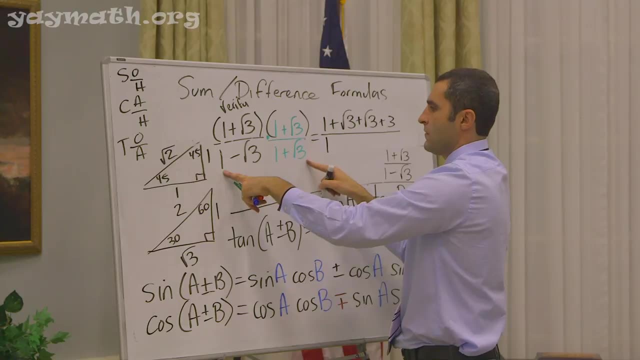 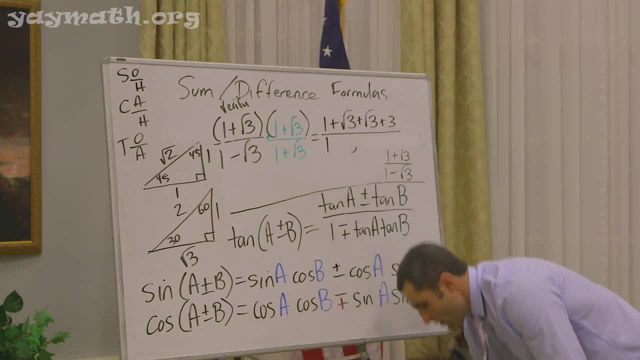 1.. 1. Outer Root 3.. Plus root 3,, that's right. Inner Negative root: 3.. Negative root 3.. Yeah, I'm going to put it in red so you can see that they're going to cancel. 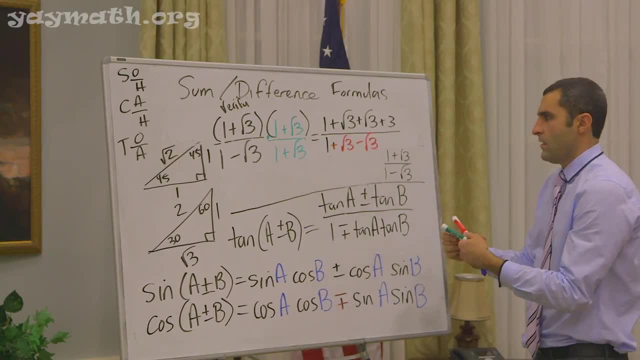 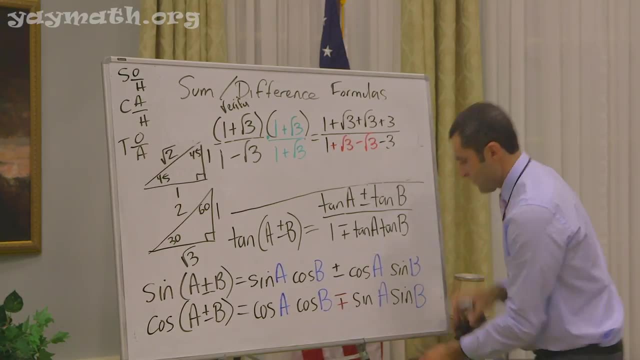 Negative: root 3 minus 3.. Good, Plus root 3.. Minus root 3.. And then we can cancel a bunch of stuff And then we have minus 3 on the bottom, And then we can, but then it's root 3 minus root 3, so we can just cancel it. 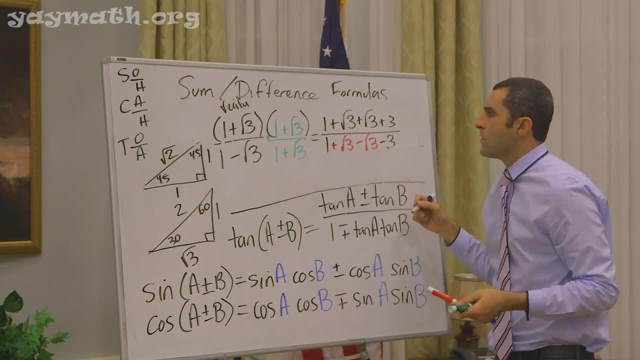 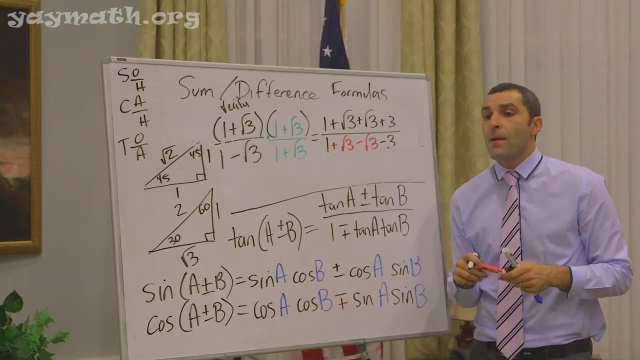 So those cancel, that's right. What's upstairs? Hook it up upstairs. The 2.. Wouldn't it just be root 6 plus 4? Root 3 plus root 3 is 2 root 3.. Oh, 2 root 3, yeah, yeah, yeah. 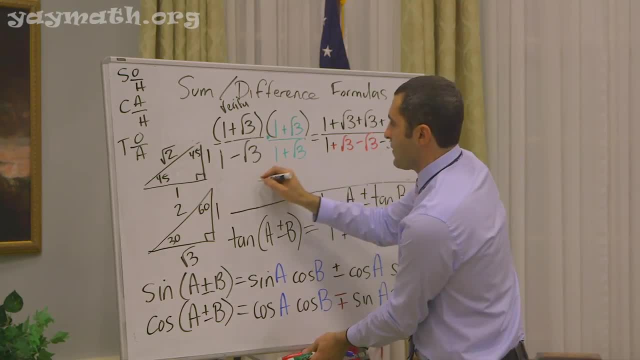 Remember they don't combine 2 root 3 plus 4.. So it'd be 2 root 3 plus 4, fantastic. 2 root 3 plus 4.. 2 root 3 plus 4, all over. 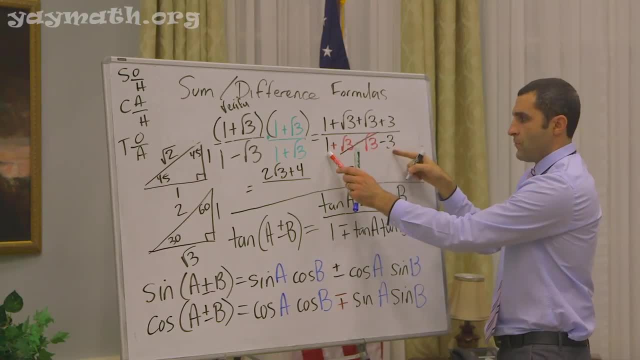 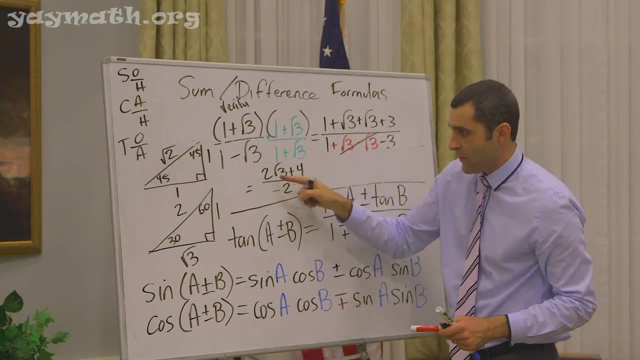 And then on the bottom it's negative 2.. Negative 2, correct 1 minus 3 is negative 2.. And then, can't that simplify? Does negative 2 divide into both terms? Yes, It does So, and then that becomes: